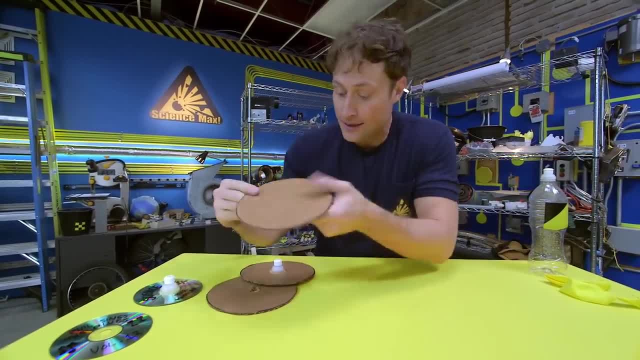 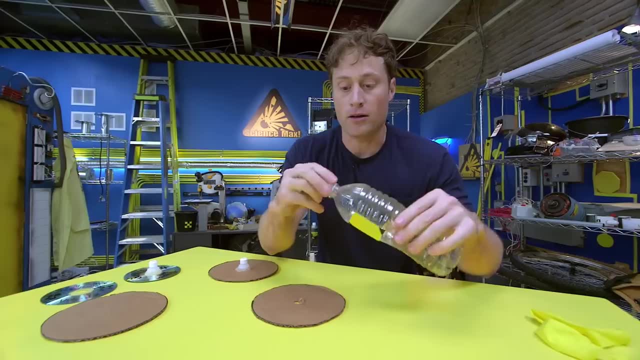 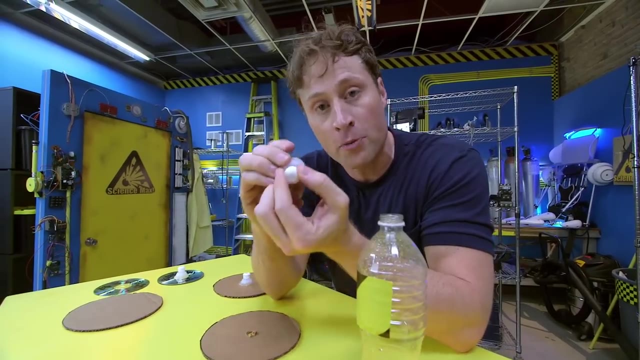 You take some cardboard and cut it into a circle just like this, Then put a hole in the middle of the circle- You might want an adult to help you with that- And then take a plastic drink bottle cap like this. I like to use the ones that you get on sport bottles because they have a little nozzle that pops open or closed. 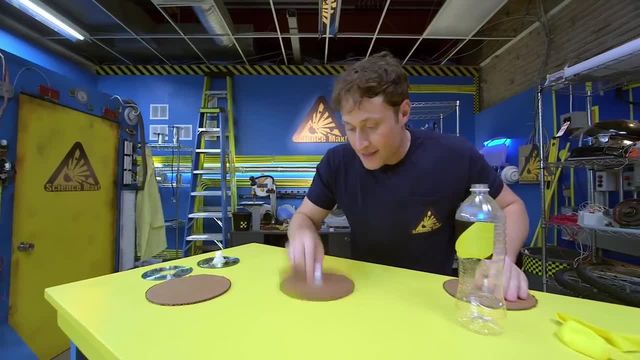 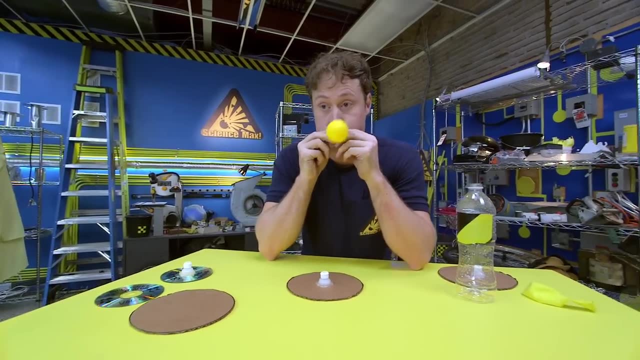 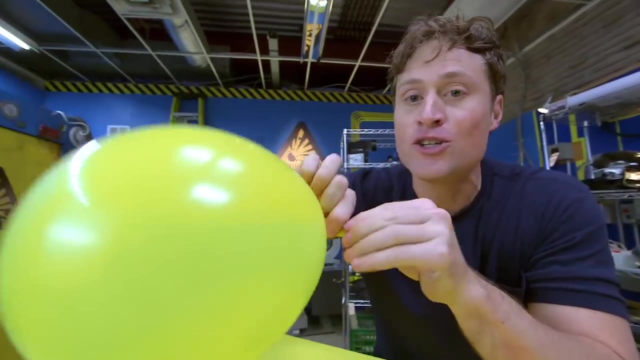 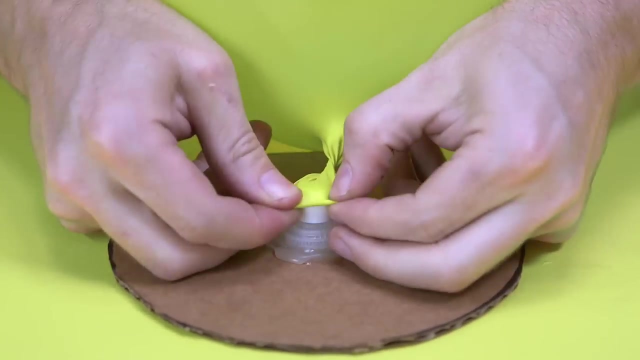 And then you glue it around the circle and you get this. Then you need a balloon. So you blow up your balloon- I know you know that step- And then twist the balloon so it doesn't get away from you. When it's nice and twisted you can stick it over the drink bottle cap, like this. 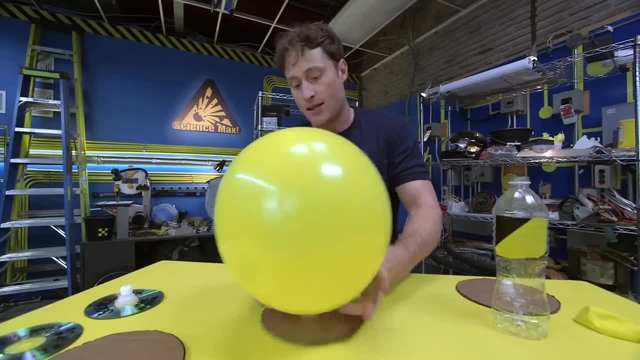 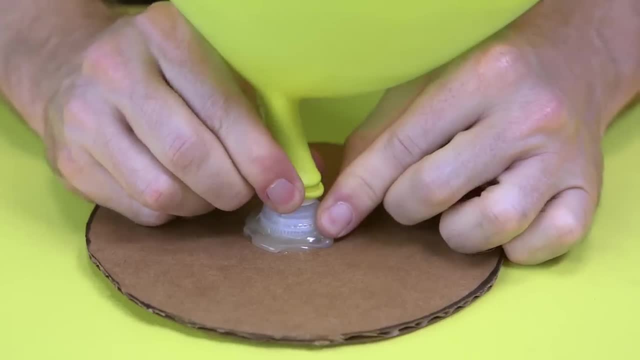 And then untwist it, And this is why I like to use the plastic drink bottle caps that come from sport bottles, Because you can open it when you want And when you do. Your disc rides on a cushion of air, reducing the friction with the table. 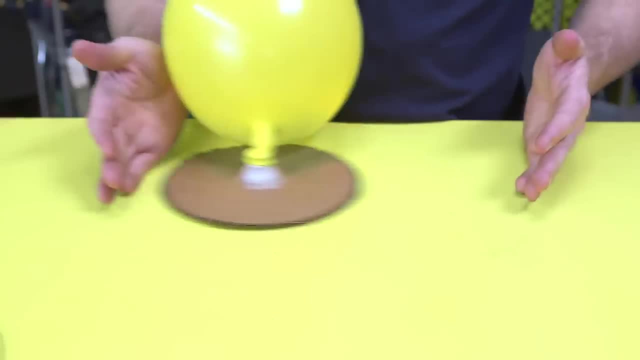 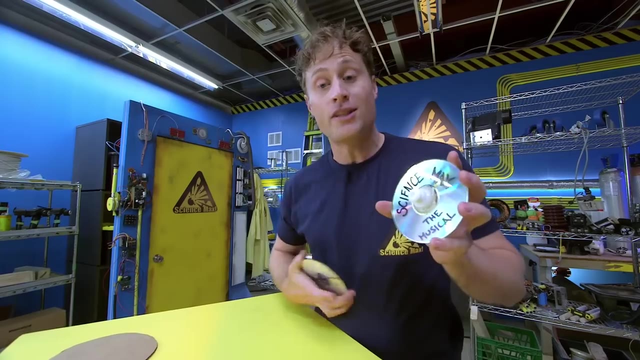 And it's almost like it's sliding on ice. You can also use CDs if you want to do a different design. Just make sure you're using CDs you never want to listen to again. Now, if any of this is too fast, don't worry. 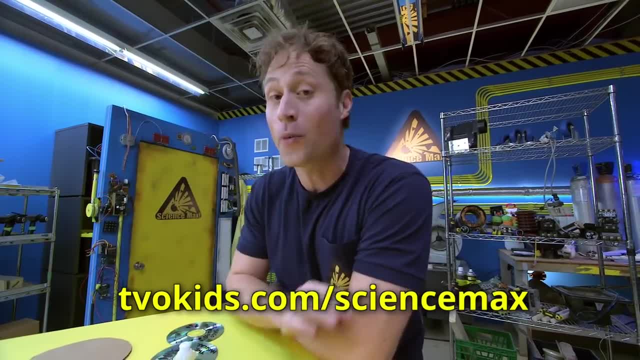 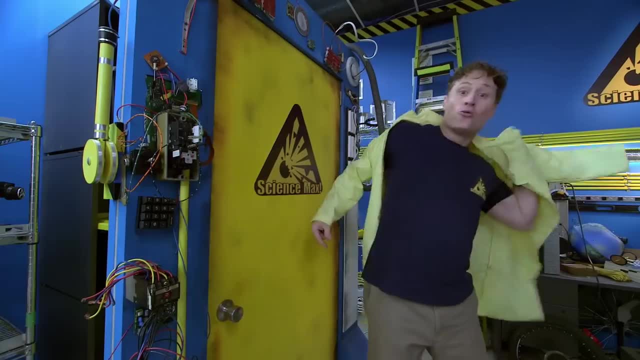 You can always go to the Science Max website where we have all of the instructions. And now it's time to max it out. We're going to see if we can make a human sign. We're going to make a human-sized, rideable, low-friction hover disc. 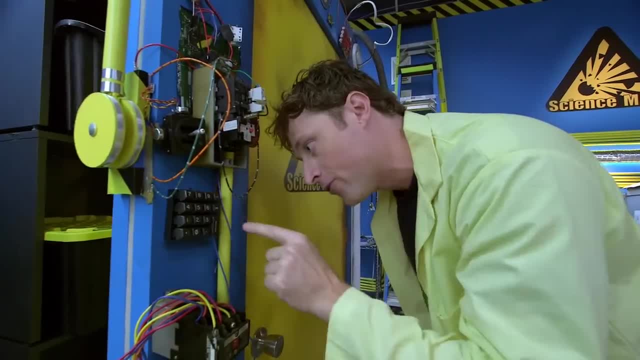 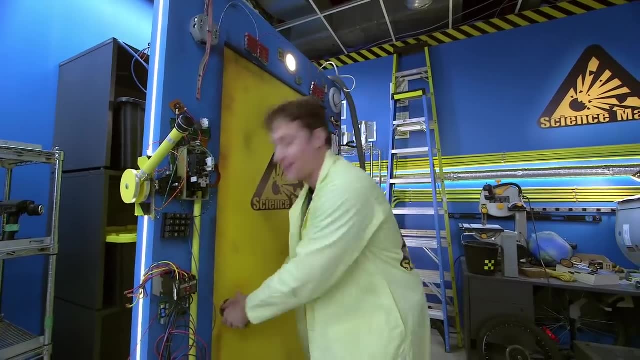 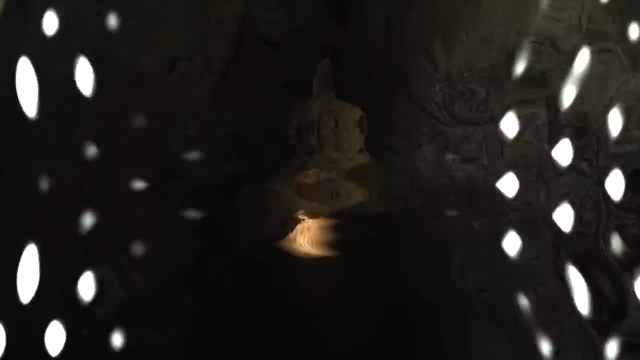 I'm going to the Ontario Science Centre where, hopefully, I have an expert that can help me. The door is stuck. I think there's a little bit too much friction with the That's got it. Oh no, This isn't the Science Centre. 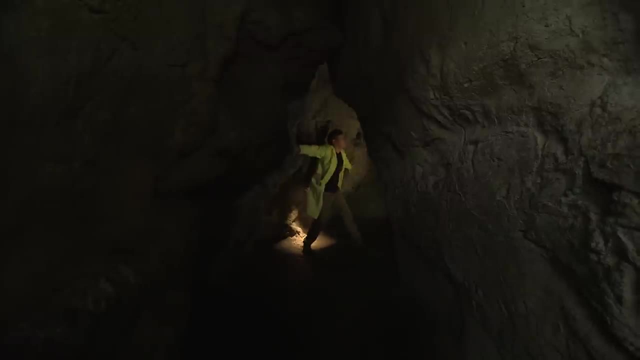 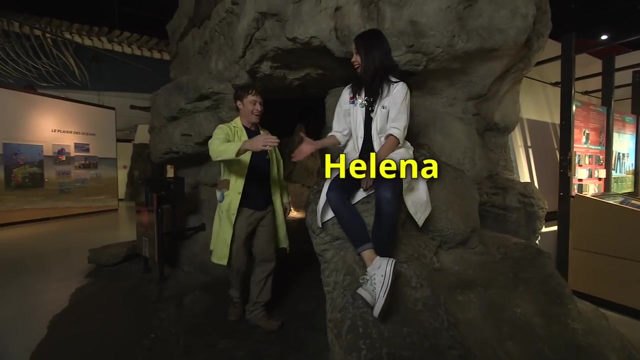 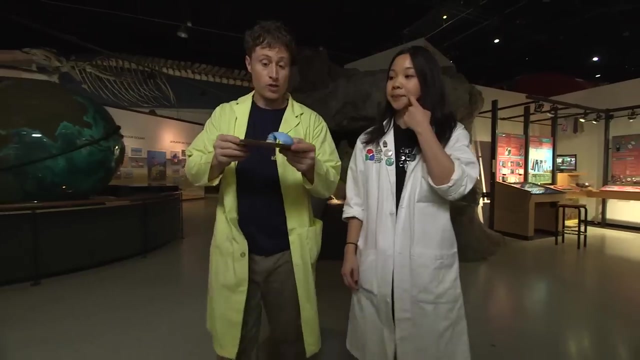 Did I go back in time again? Oh, It is the Science Centre, Helena, hi. Hey, Phil, You're here to see the hover disc. Yes, please, Alright, come on Right this way. So I made one in the lab. that works pretty great. 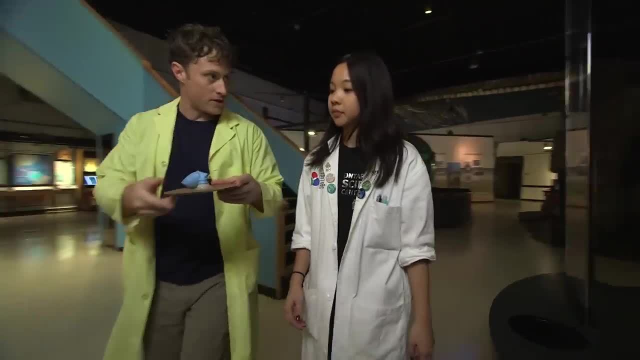 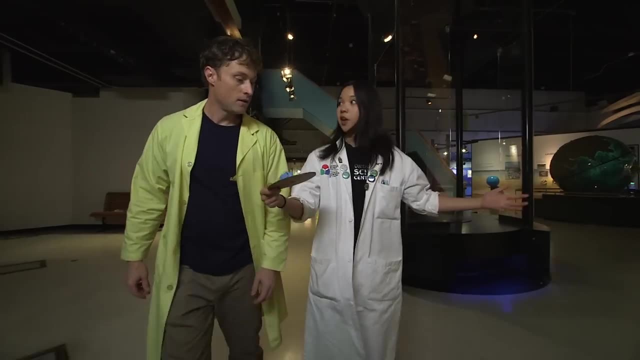 It's on cardboard and it has a balloon. The one you have here works on the same principle. Yeah, it does. But you know what? My friend Russell has some ideas about making something like this, but even bigger. Do you think we can make one big enough to ride? 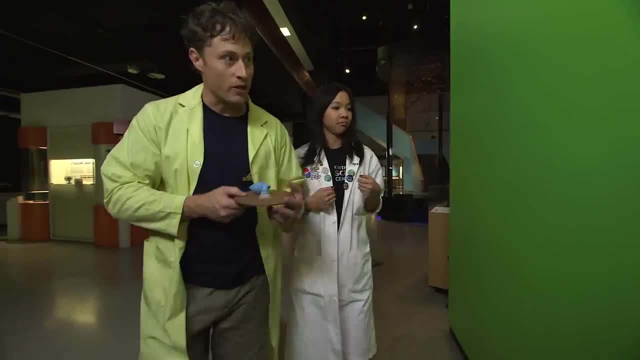 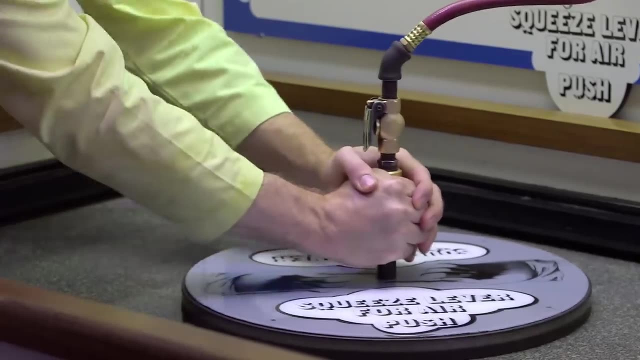 Maybe, yeah, Alright, well, let's take a look at the one you have here. Oh, I see, Right, this one works the same as the one I made. It's really hard to move the disc, but if you add some air it floats like a dream. 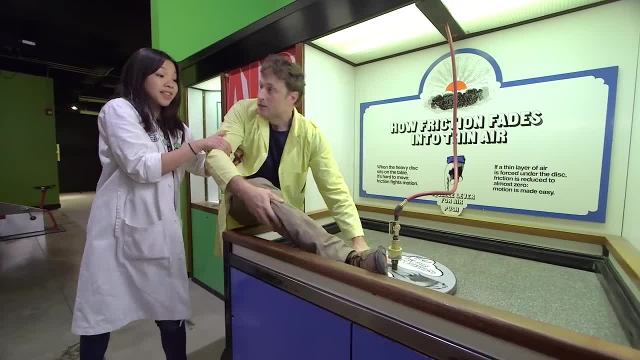 There we go. Great, so let's ride it. Whoa, Phil, Not this one, the one upstairs? You can ride that one. Oh, okay, Yeah, Should we bring this one? No, that's a little heavy. I think we can leave it there. 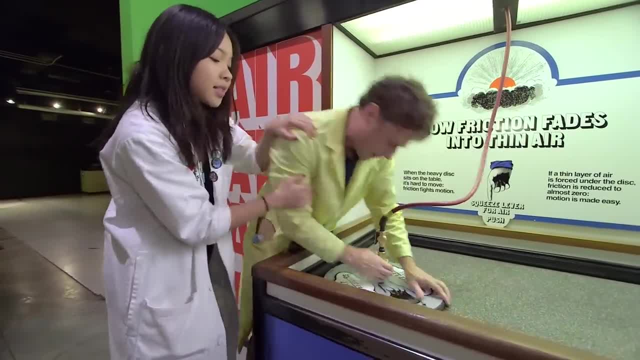 What if we need it for reference? No, I'm sure we'll be okay. It is pretty heavy. Yeah, come on, Let's go. Russell's waiting. Are you sure we won't need it? I'm positive. No, you have to come back. I get to say I told you something. 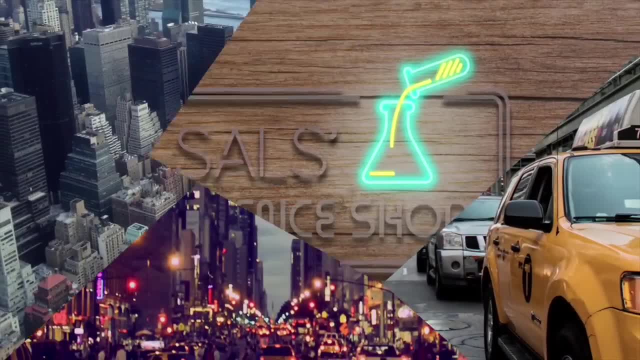 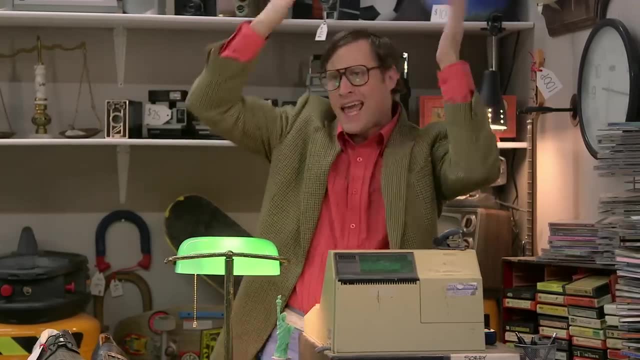 Okay, Alright. Hey, Ramona, You ever change your hair. Yeah, it's nice, It's like doing this now. It used to be, but now it's. yeah, I like it. You should give me the name of your guy. 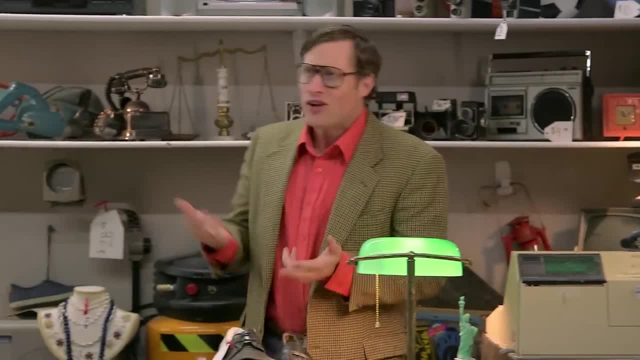 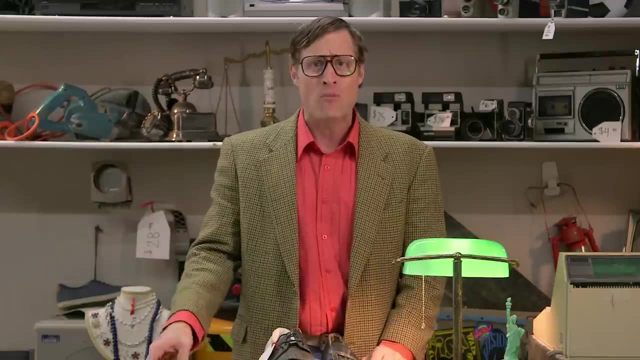 because I wanted to. oh hey, how are you? You ever think to yourself: no matter what I do, I can't seem to get anywhere, I can't get enough traction. Well, you, my friend, need some more friction. 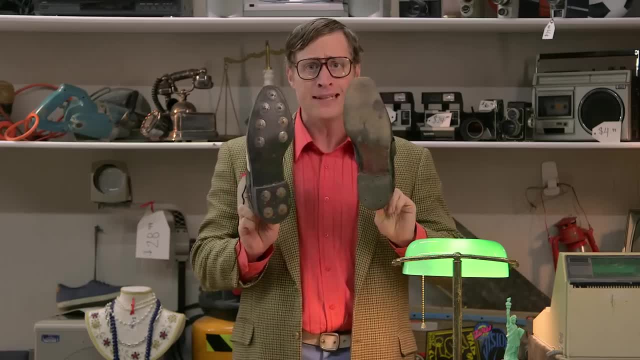 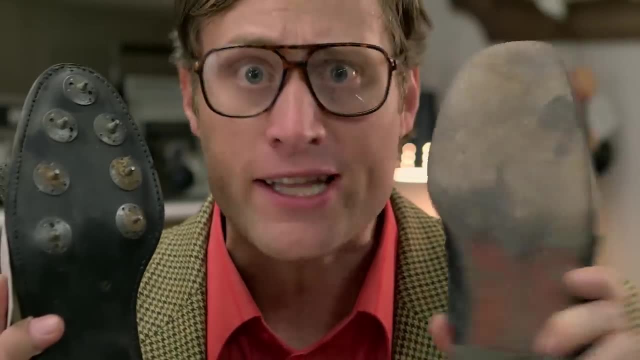 Which one of these two shoes has more friction? Hmm, Let's take a closer look. Huh, Huh, Right, Bam. This one. This one doesn't have a lot of treads, It doesn't have a lot of friction, But this one, it's got metal spikes on the bottom. 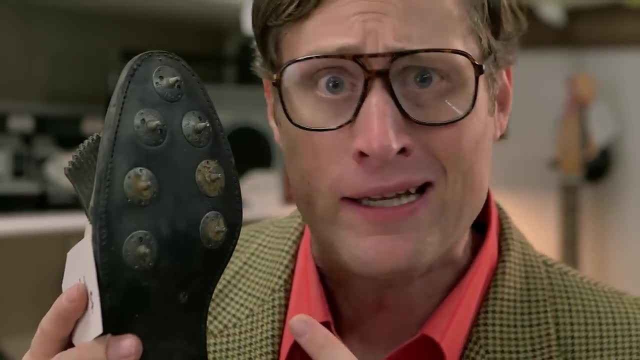 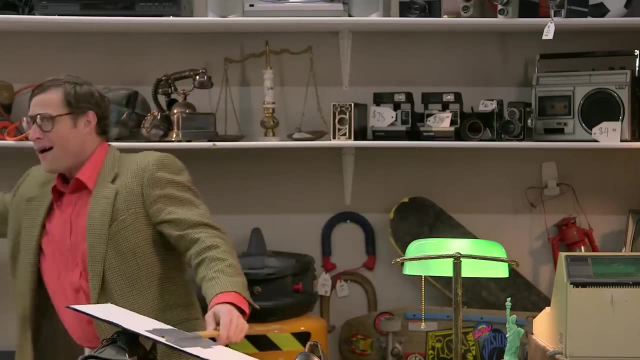 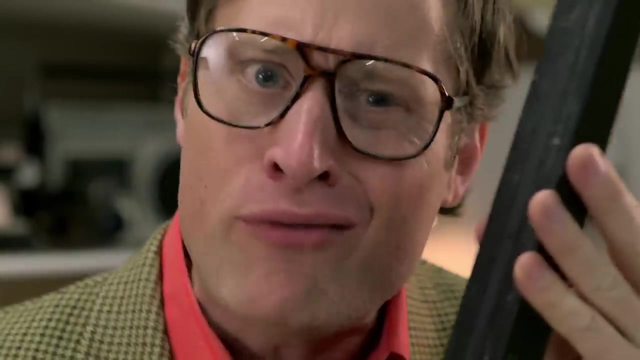 This is called a cleat, and the spikes are for helping you grip onto the grass when you're playing soccer or golf, increasing its friction. Why do you think skis are smooth on the bottom? Come on, Look at that. It's so smooth and glidy. My hand just- I can barely even touch the surface. 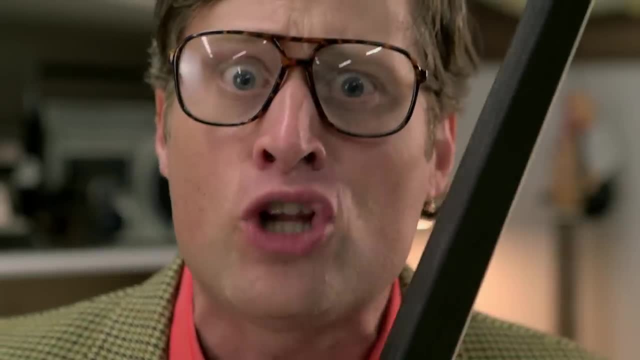 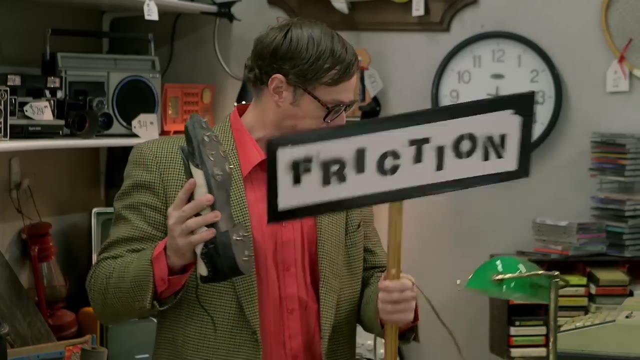 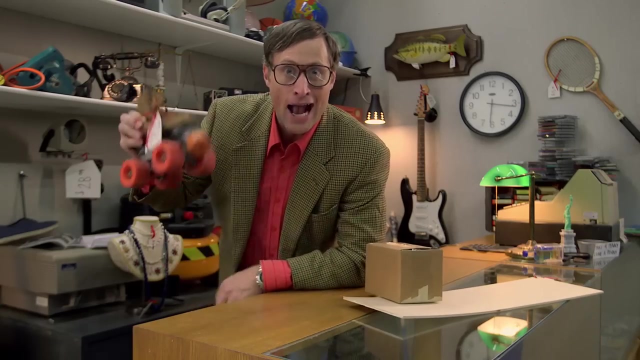 It just slides right off. It's sort of glidy and smooth. They're smooth to help you glide across the snow, reducing their friction. Why doesn't this box slide down this ramp Friction? This roller skate has wheels. Wheels reduce friction. 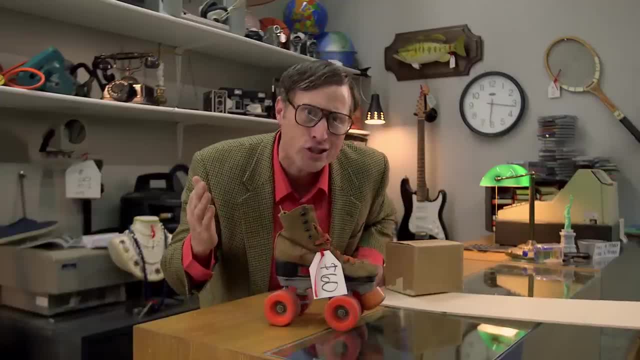 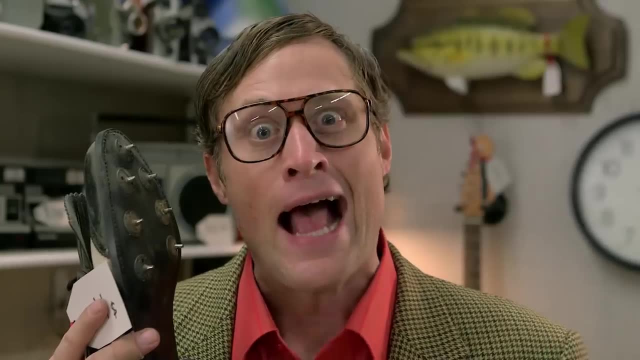 But when I push the roller skate, how come it doesn't just keep rolling forever and ever and ever and ever, and going all the way around the world and writing a memoir? Say it with me. Friction, Louder Friction, Can't hear you. Friction, A little too loud Friction. 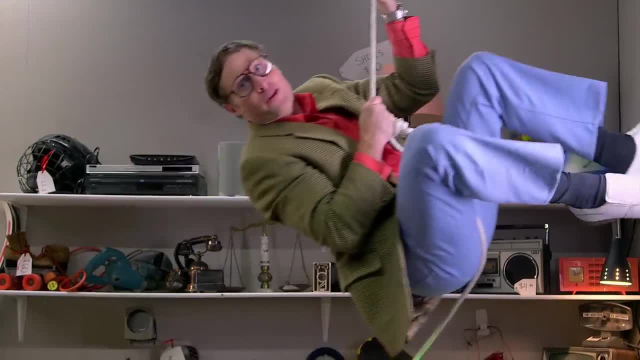 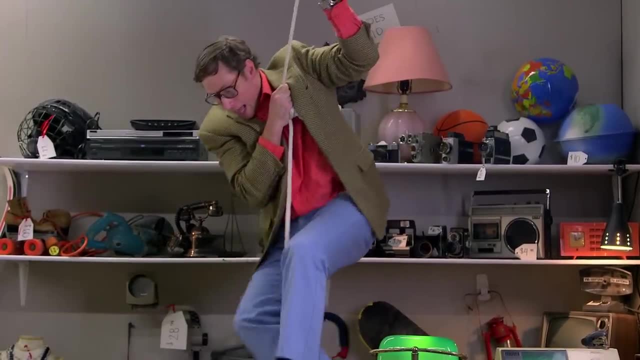 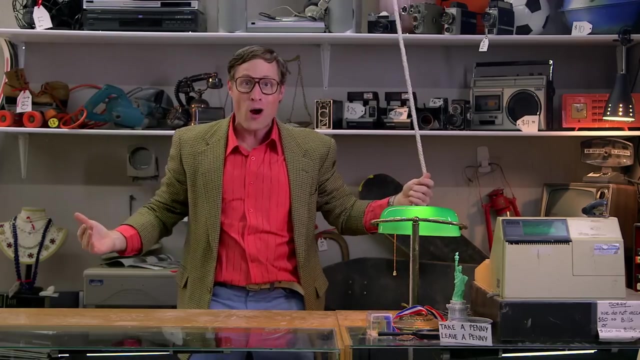 Ease it back, Friction. How can I hang onto this rope without falling Friction? How can I? How can I jump down on the floor without falling over Friction? And now you know: your friction, Your friction, You. 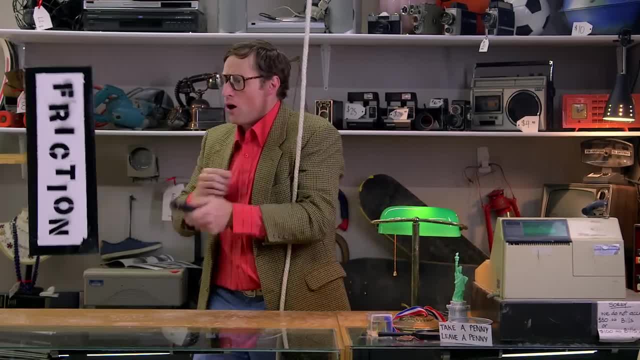 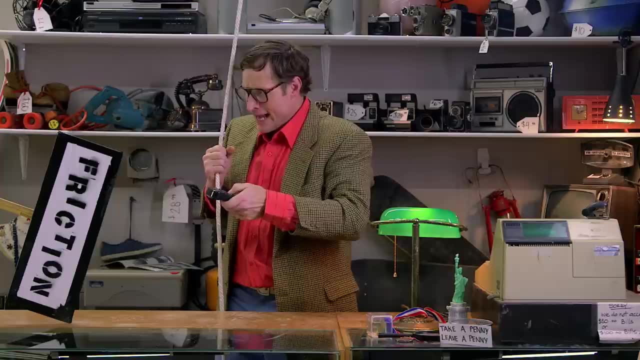 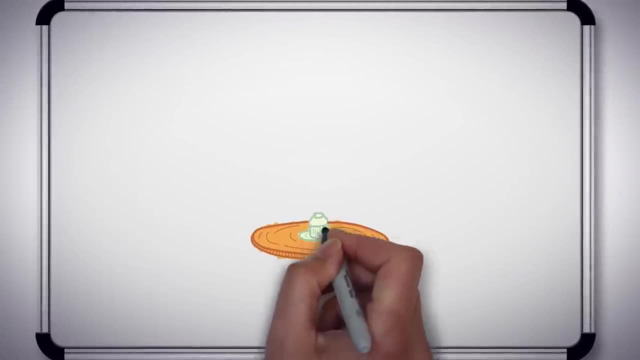 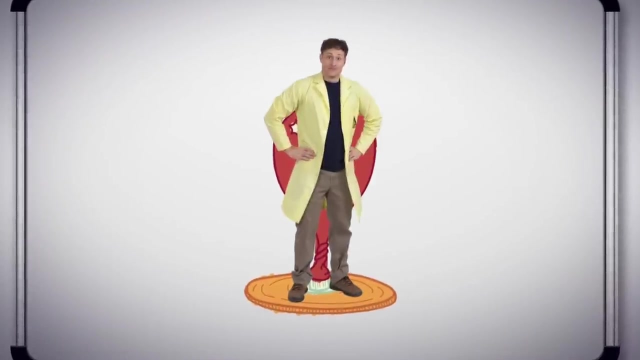 Your friction. Come on, Uh-oh. Oh, Ramona, the friction sign is broken, Reset, Uh-oh. The plan is to take our small hover disc and make one big enough to ride. So I'm off with Helena to another part of the Science Center to meet Russell, who has some ideas on how we can do it. 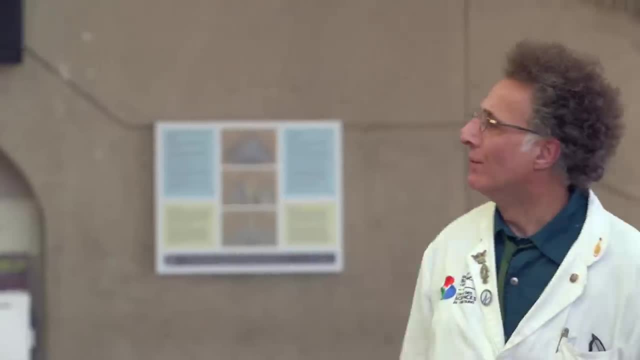 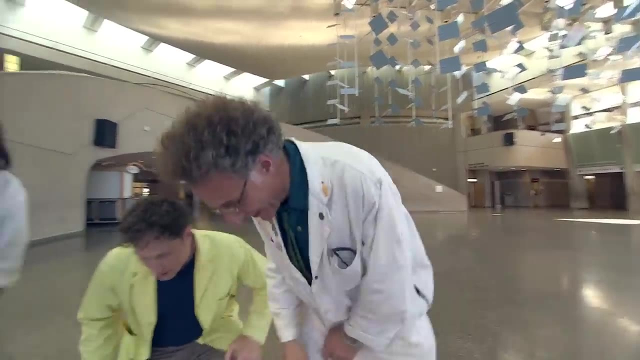 Oh, hey, Russell, Hey hi Helena, Hey Phil, How you doing Russell, How you doing Phil? So this is the hover disc. This is our small hover disc. yes, How does it work? Well, um, obviously you sit on here. 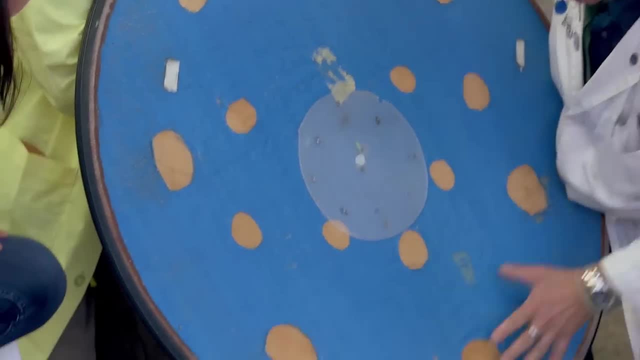 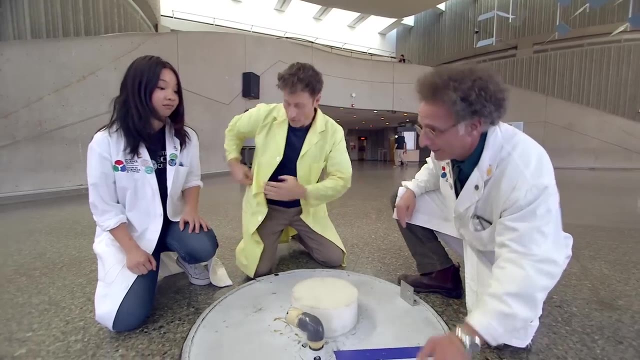 Right, Air will go into here. It gets vented through all these separate holes here, so we get an airflow over the entire area. Hopefully this will work. to pick someone up, All we need is Air. Oh well, that's easy, because the small one works like this, so I'll just 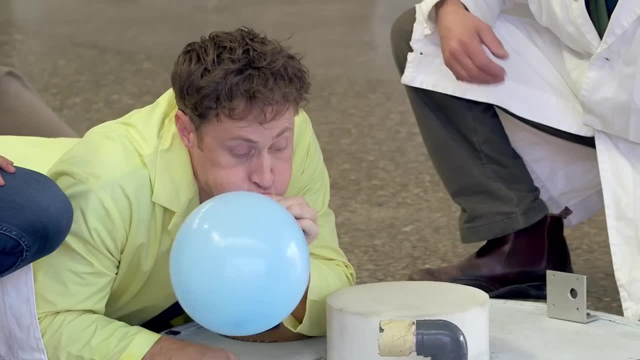 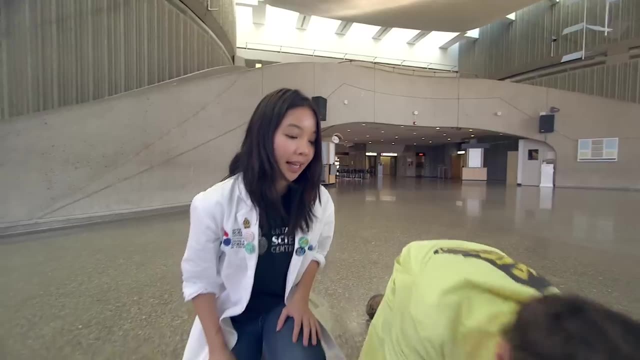 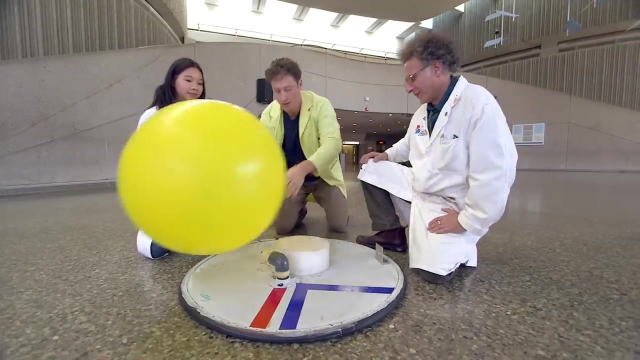 We just put the balloon on right. Uh, Okay, so we put the balloon on the Uh, hold on, hold on, hold on Larger balloon. Okay, Sorry, sorry, That's okay, Okay, Uh-oh, twist it so it doesn't. 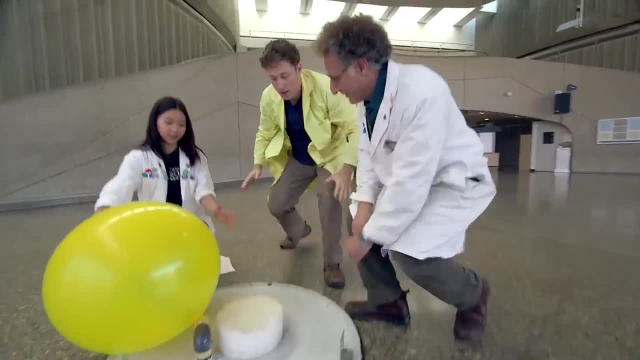 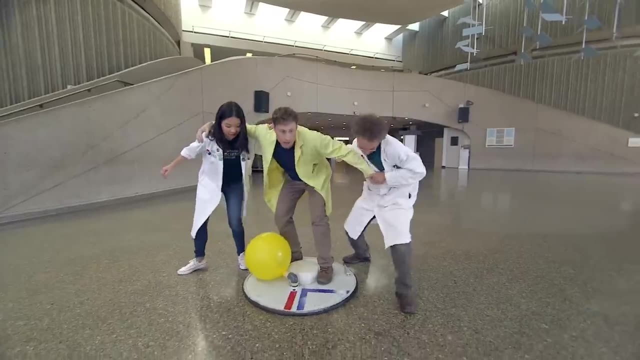 He's losing his hair. Okay, All right, On again. Hold on, You grab one side, I'll grab the other. Okay, Here we go. Go It's not. It doesn't feel way too much friction on that. 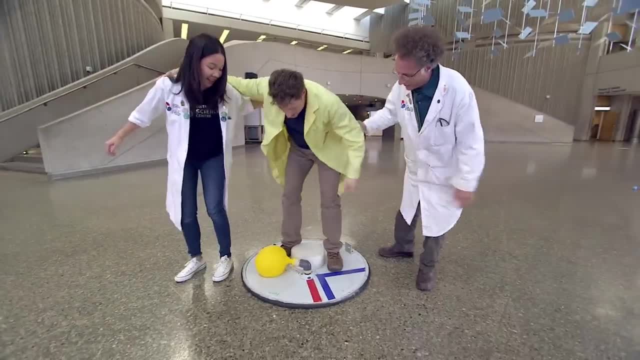 It doesn't feel like there's, There's, uh, It still feels pretty frictiony. I think, uh, I think we might need something more than a balloon. So what do we do? Well, I think we need more consistent air going through here. 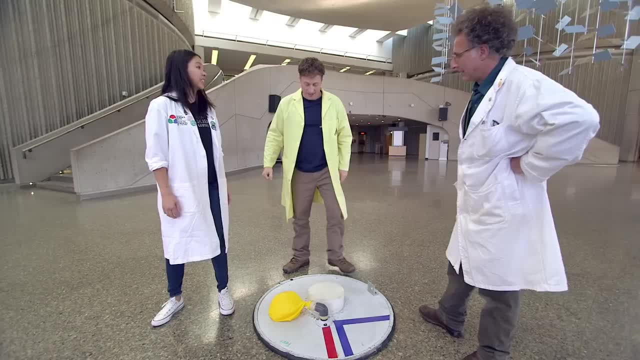 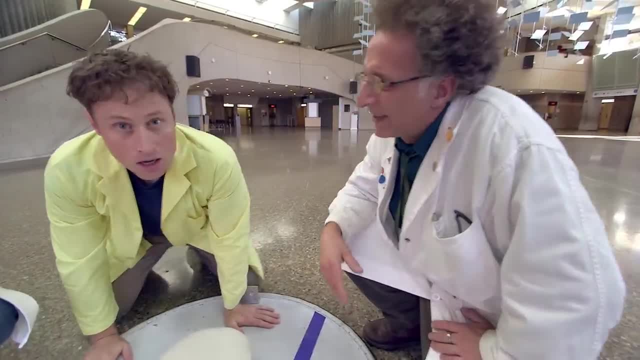 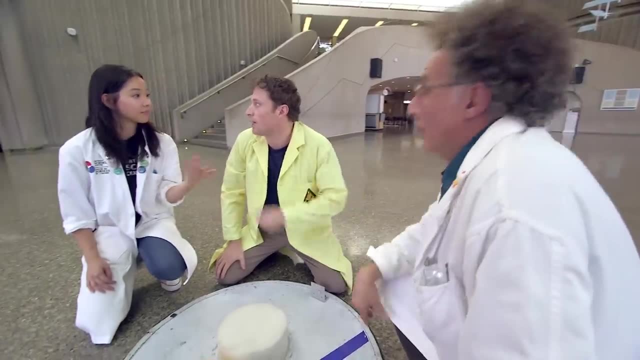 Opposite to a vacuum cleaner. Yeah, Opposite to a vacuum cleaner. Yeah, Opposite to a vacuum cleaner. Opposite to a vacuum cleaner. That would be a Like a leaf blower. Like a leaf blower, A leaf blower. 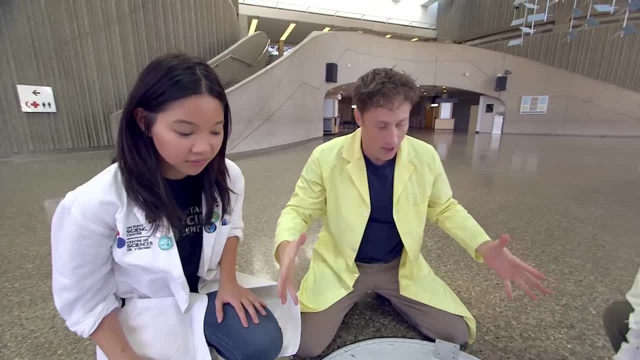 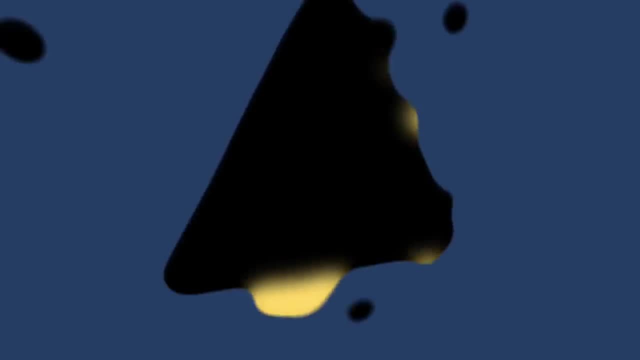 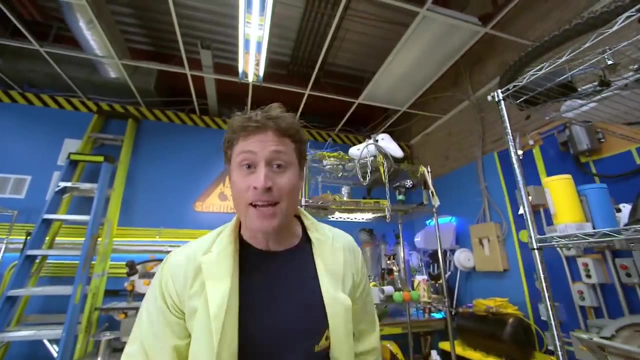 High five. Yeah, Awesome idea. So why don't we make a couple larger discs and we'll hook some leaf blowers to them and we'll see what happens? Definitely give it a go. Okay, Great Carbon is an atom and is the basic building block of all life as we know it. 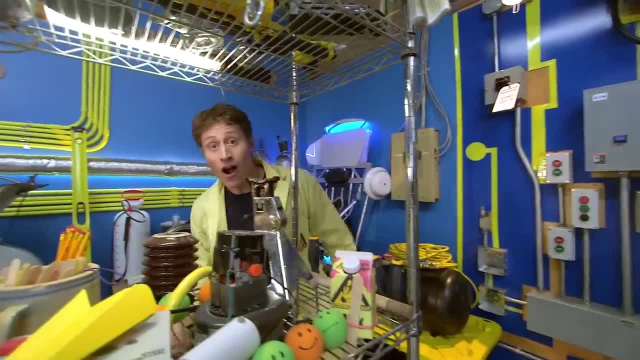 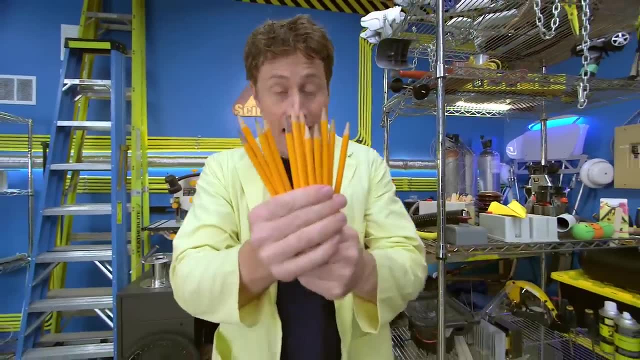 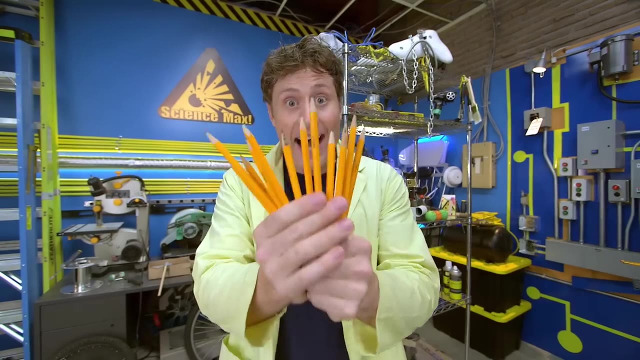 You, me, all plants, All animals are carbon-based life forms. Other things are made of carbon too. Diamonds are carbon, coal is carbon, even pencil. lead isn't lead, it's graphite which is carbon. If you were to take all the carbon atoms in your body, you could fill 9,000 pencils. 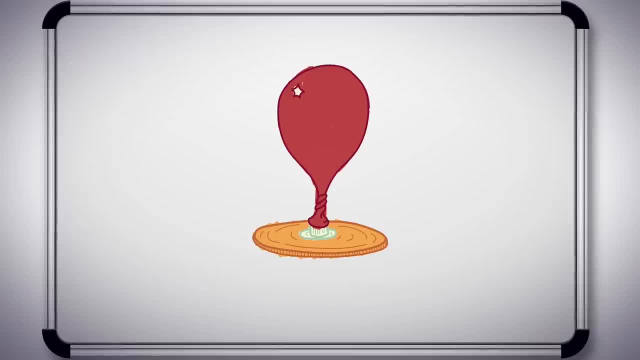 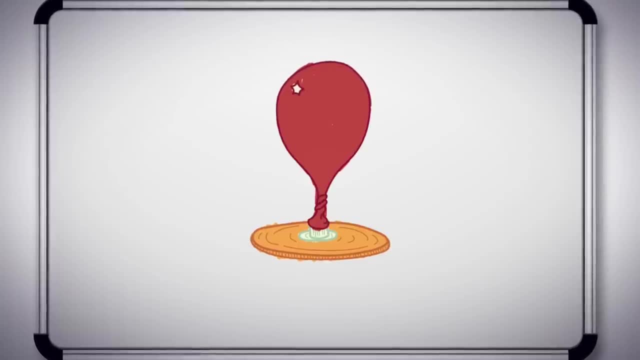 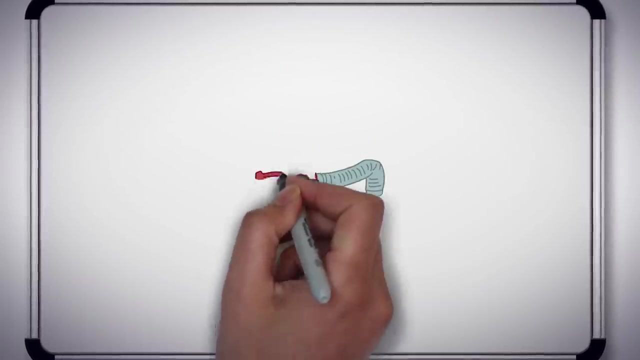 Of course I kind of prefer my carbon where it is. Our low-friction hover disc still had way too much friction. One of the problems that Russell mentioned is that the balloon. The balloon just wasn't giving enough air, But then Helena had the idea of using a leaf blower instead. 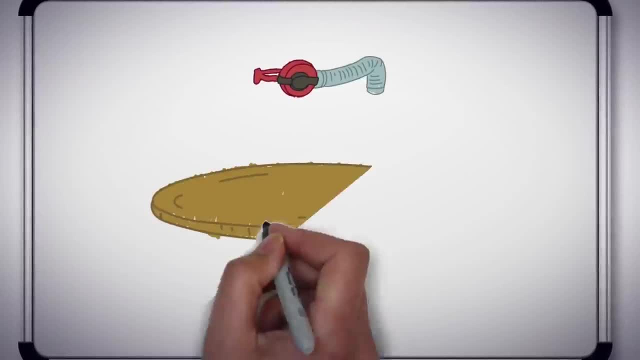 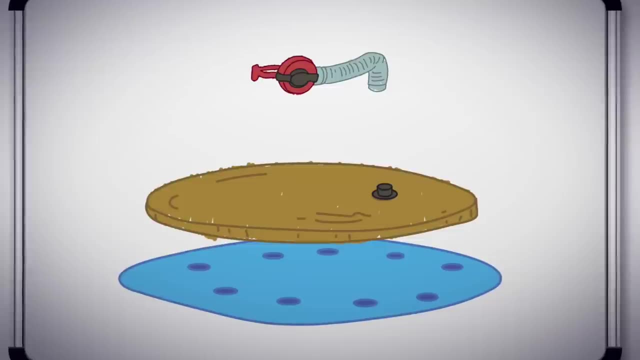 The plan now is to make a leaf blower power disc by starting with a big circle of wood, cutting a hole in the wood where the air will come through, and then covering the bottom with a tarp that has many holes cut out of it for the air to escape. 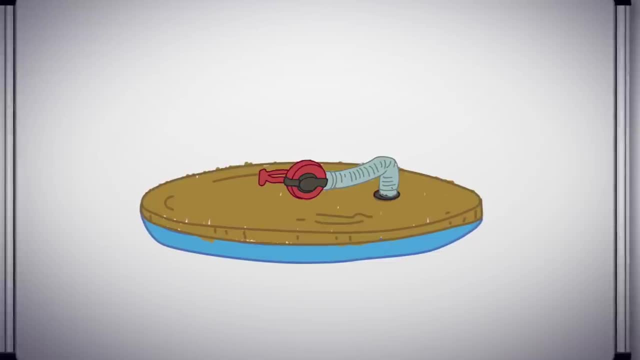 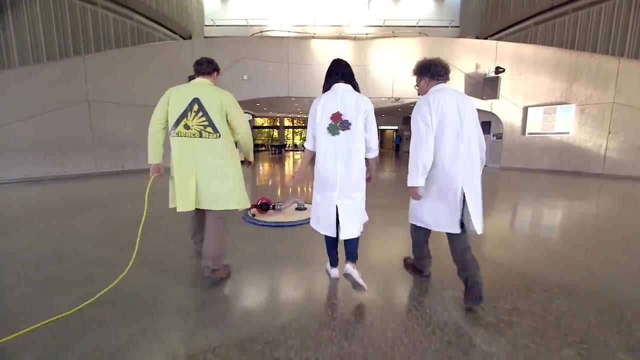 Because leaf blowers are made to push lots of air. hopefully they'll be enough for me to ride it. Well, this is the business. Look at this. That's amazing. It's good, right? Oh yeah, I love that tube. 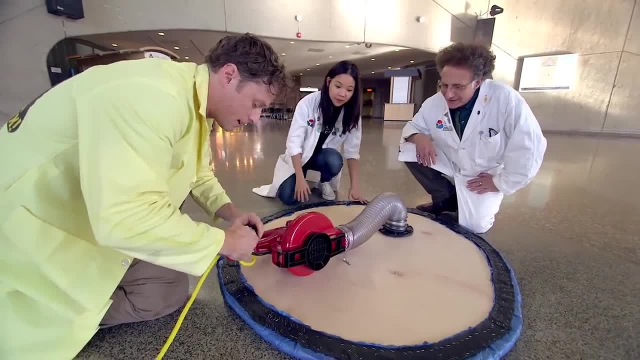 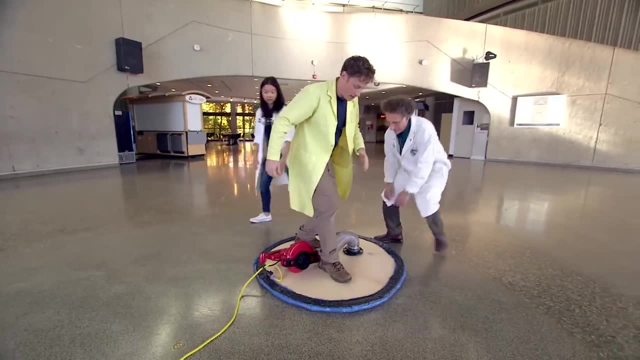 High volume of air through that. Yeah, So, yeah, I think it's a dryer vent, that I just found it in the lab. And then this, of course, is a leaf blower, So I get on here and then, Helena, if you want to turn it on, 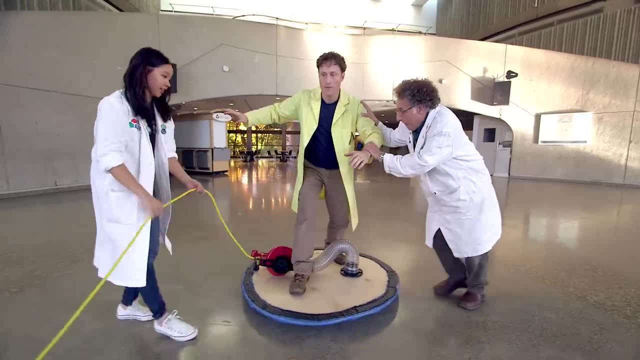 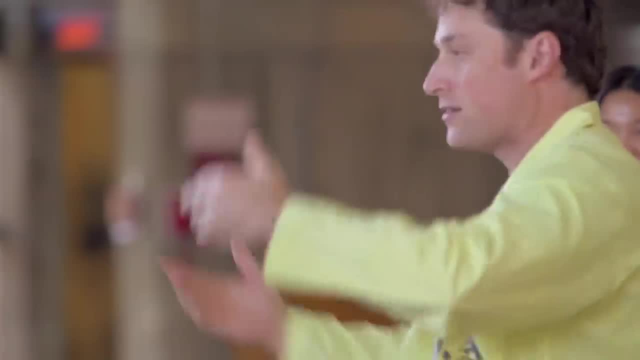 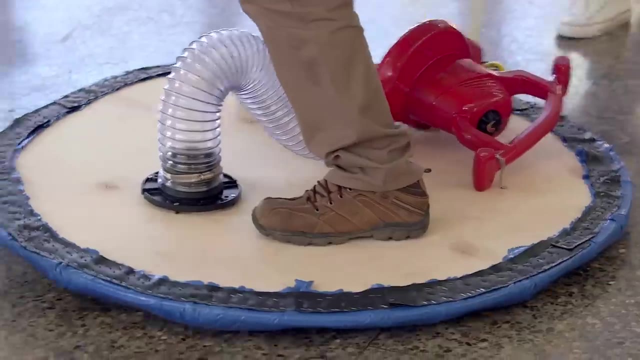 Yeah. So once we fire it up, the air coming out from the bottom of the disc raises me up and I float on a cushion of air. I can't control it Because the friction between the disc and the floor is so low. I end up floating wherever. 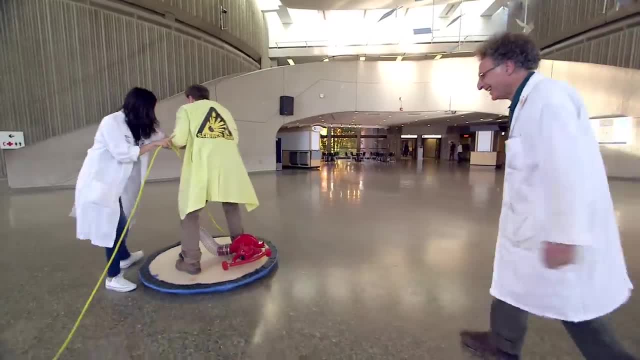 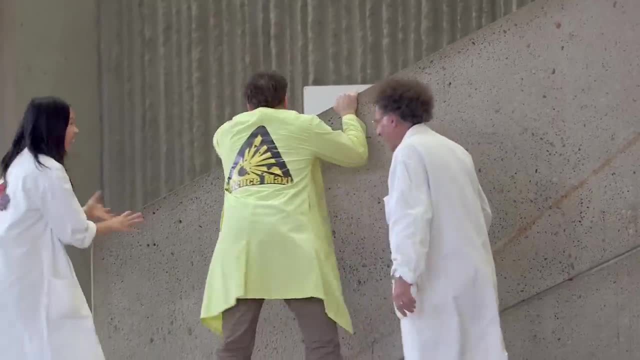 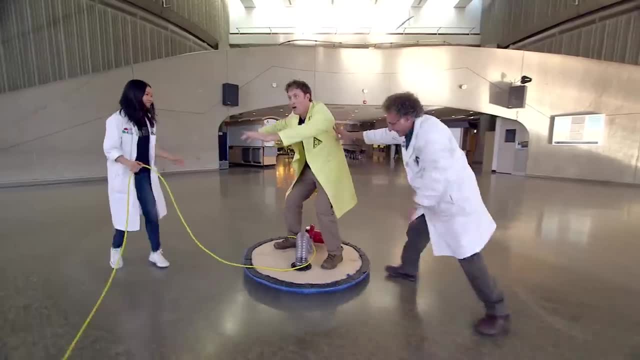 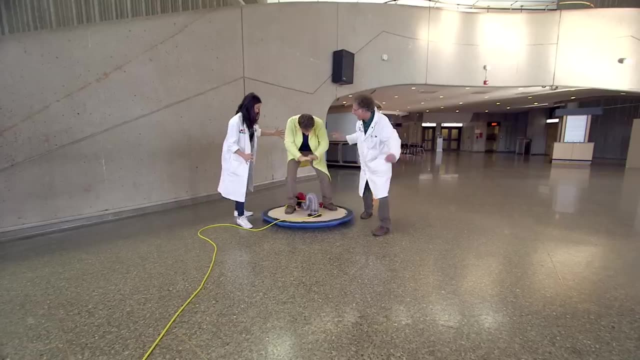 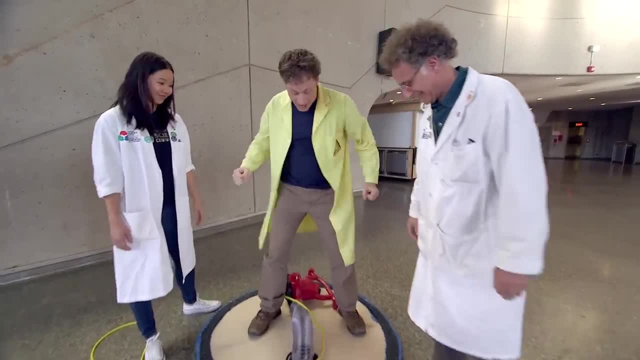 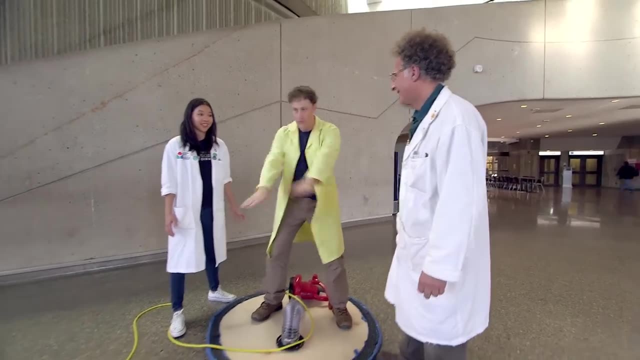 I have no control whatsoever. Yeah, no, But this is great. So we have the no friction down pat. I feel we need some way to actually move, Well, something to push you along. I was thinking, as you were going, like you need like a broom or something. 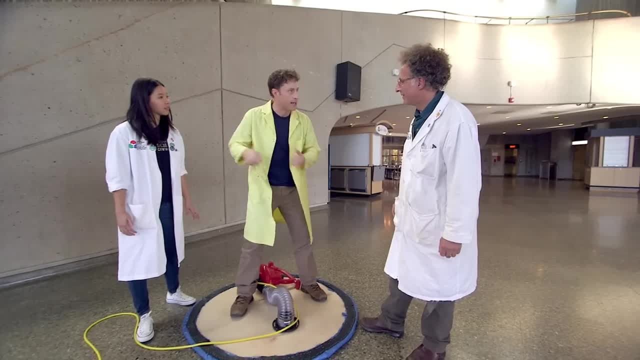 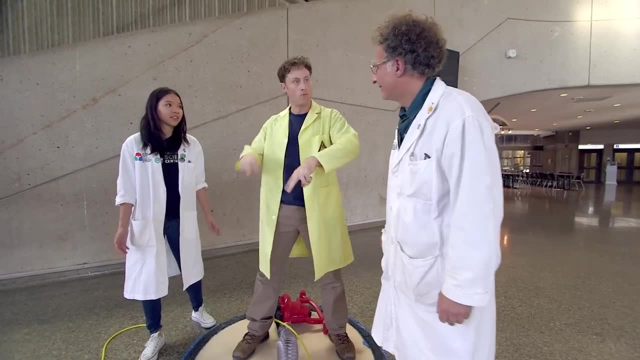 A broom. okay, yeah, What if we do like something low friction like a broom and something high friction like that? we could really sort of stick on the ground, Yeah, And then we could build two of them and we would have two discs and two ways of moving them. 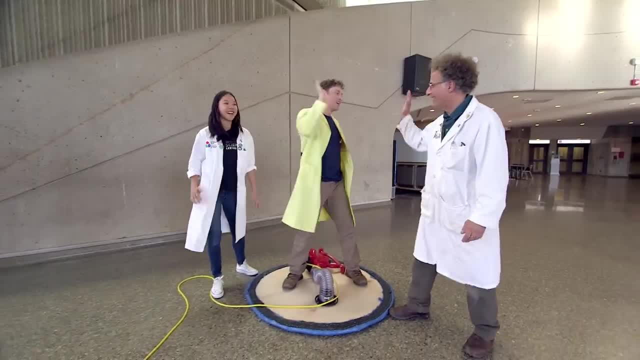 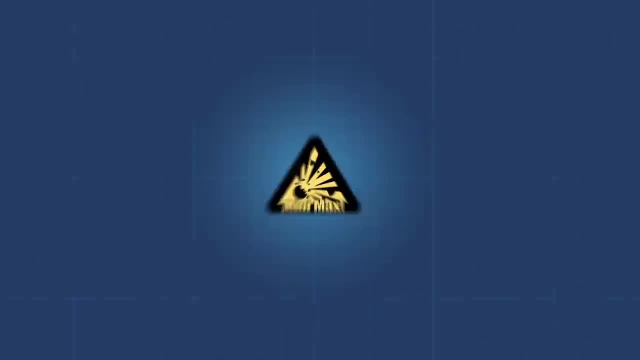 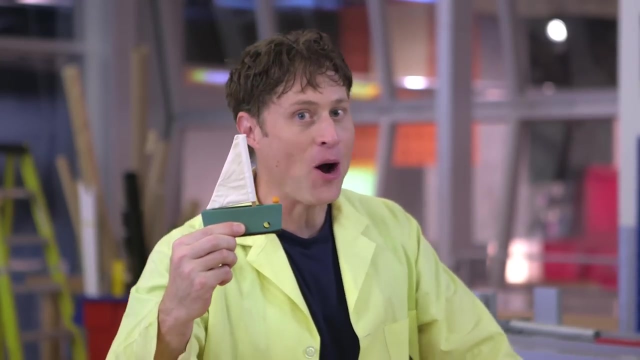 Are we gonna race? And we can race, Yeah, okay, that's what we're gonna do. Here is an experiment you can do at home with friction. This is a toy boat- Yes, you guessed that right- And this is a wooden plank. 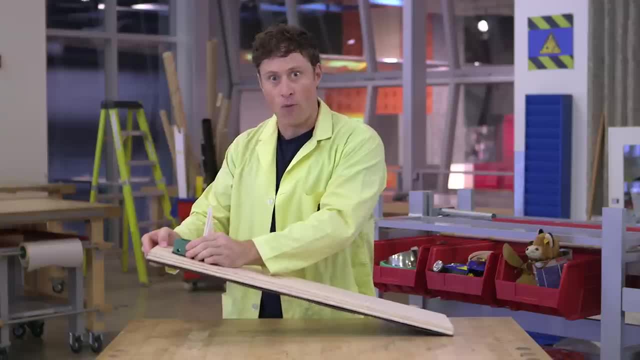 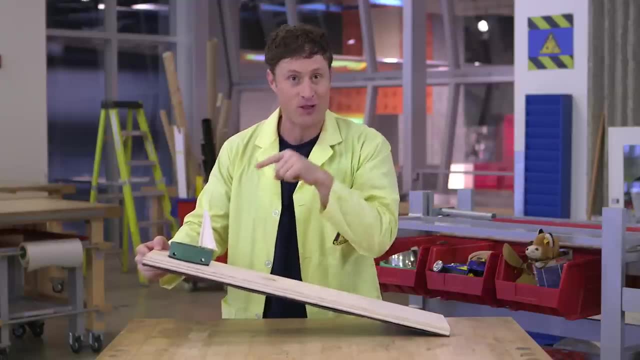 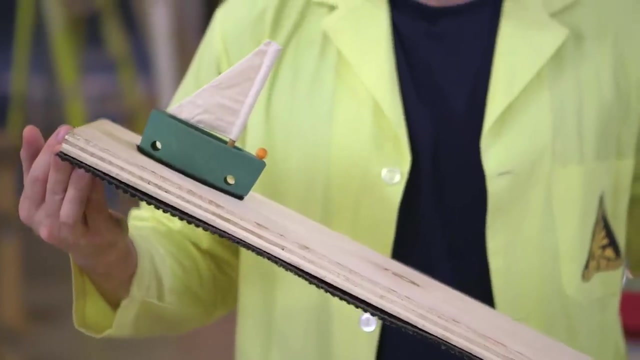 Correct, that's two for two. I put the boat on the ramp and watch what happens- Nothing. The reason why is because the friction between the boat and the ramp is enough to counteract the force of gravity trying to pull it down, But watch what happens if I raise the ramp. 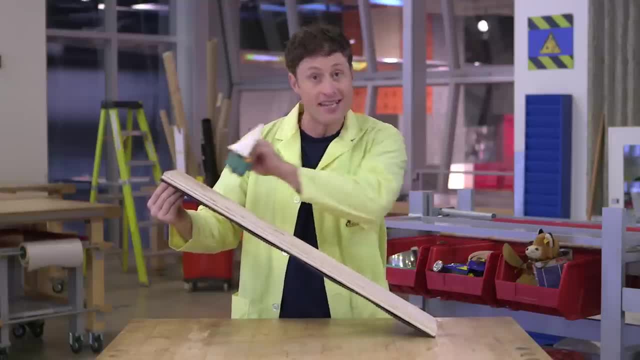 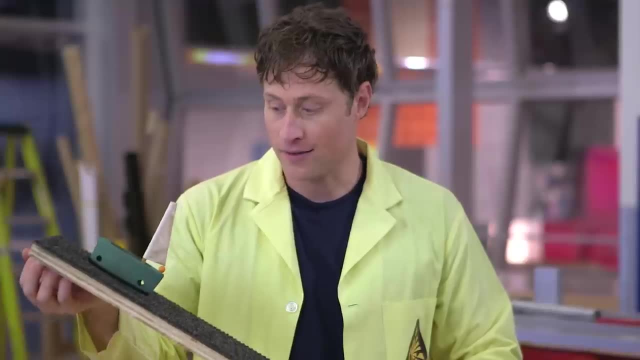 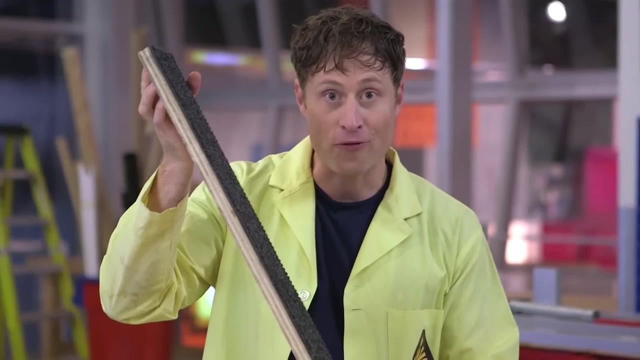 to the right height, the boat slides down because the friction isn't enough and gravity pulls it down. But when we change surfaces to this carpet, let's see what happens. Same angle: I can raise it higher, higher, higher, because there's more friction. 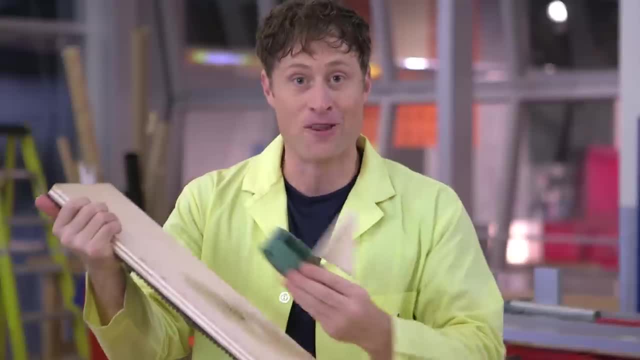 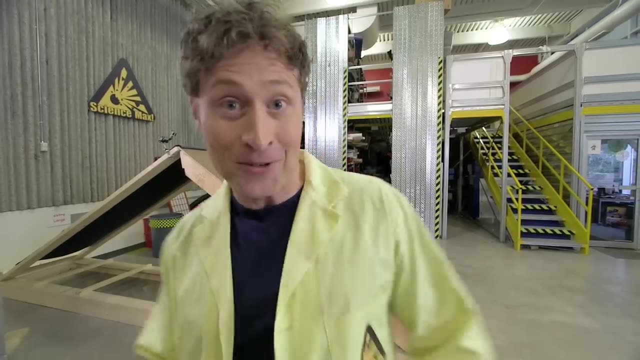 between the carpet and the boat than there was between the wood and the boat. Now, if you're thinking that we're just gonna do it with a small ramp, you're wrong, Because of course we're gonna max it out, Hey, Helena. 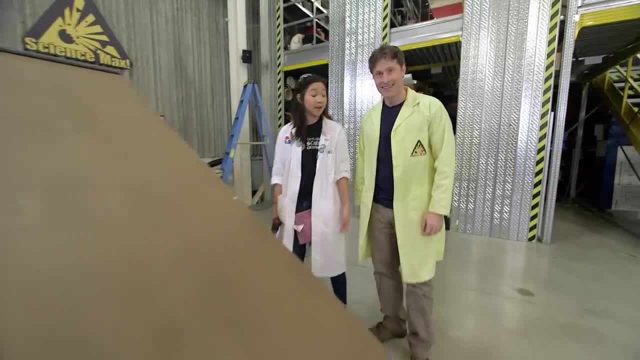 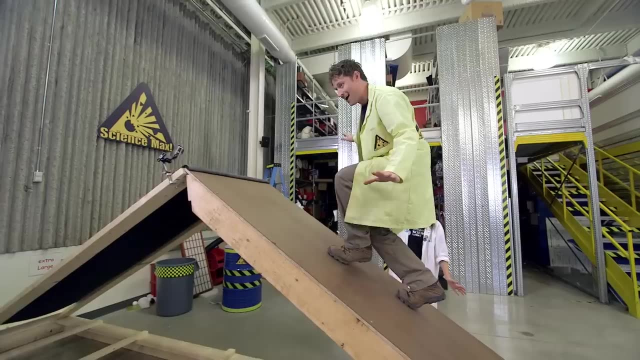 Hey, This is amazing. Thanks, I made it myself. Wow, Ready to climb it, Absolutely, Here we go, Mm, Mm, Mm, Mm, Mm, Way to go, Huh, Huh. 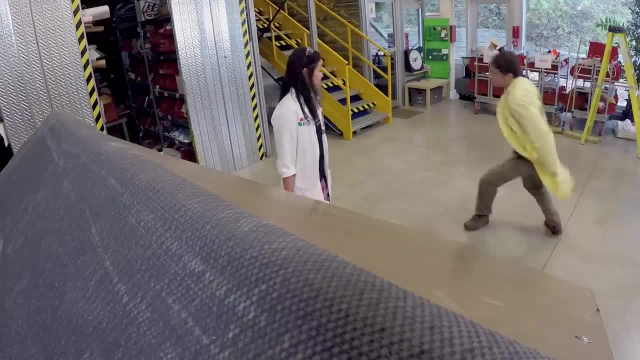 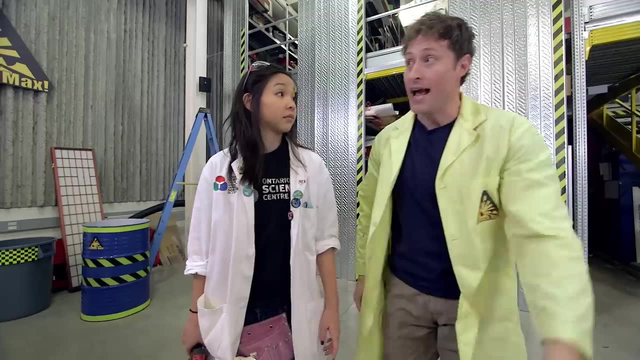 No problem. So that was very easy. Well, that's probably because the friction from your shoes is high enough so you don't slip Right, And the friction from my clothes is much lower, which is why I could slide down Right. 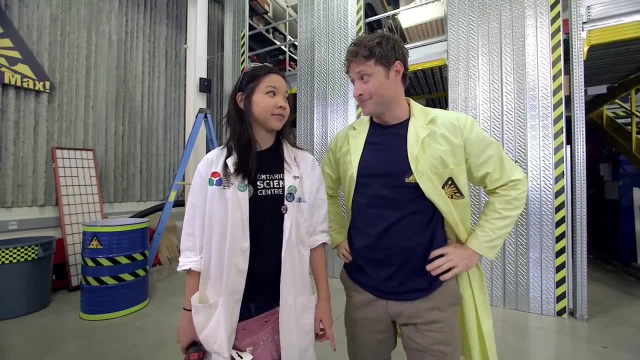 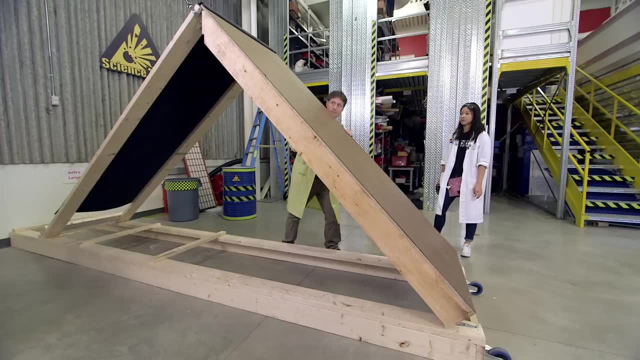 So how do we make it more difficult? We probably have to make it higher. All right, Let's make it higher With the ramp at a steeper angle. I'll need more friction to climb up. All right, Ready, I'm totally ready. 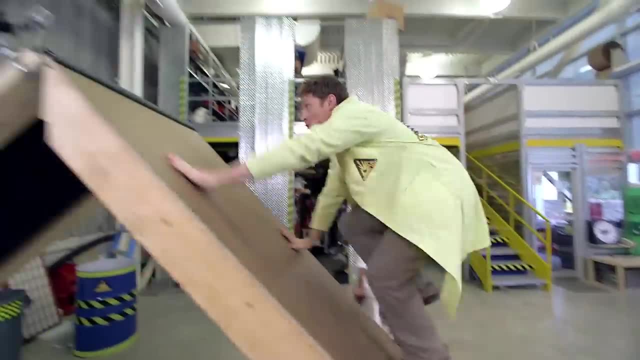 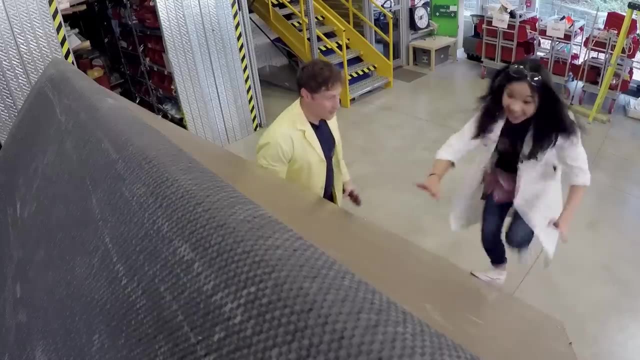 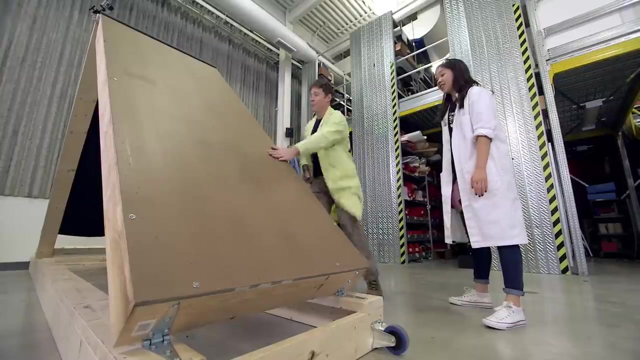 Here I go. Whoa, Whoa. All right, You try. OK, Hold my enter. Here we go. Oh, Whoa. So clearly we are not getting enough friction between our shoes and the ramp. at this angle. We should add some carpet, because carpet. 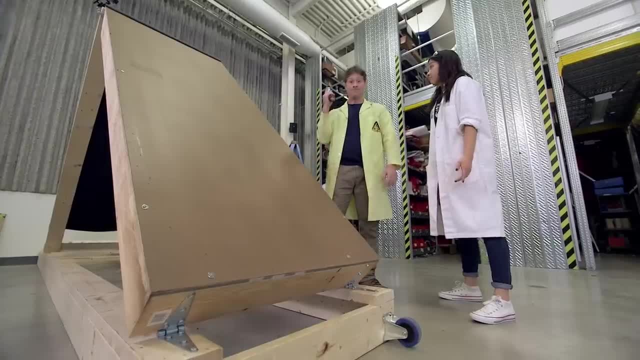 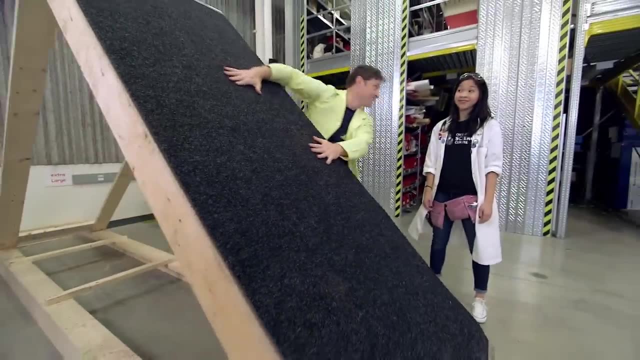 would add some more friction between our shoes and the ramp. All right, Let's add carpet. Sorry, Here's your drill, Thanks, All right, Carpet, Yeah. Same angle, Yes. And why have we done this? More friction. 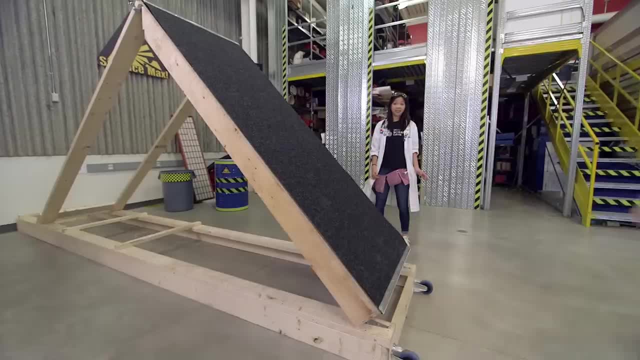 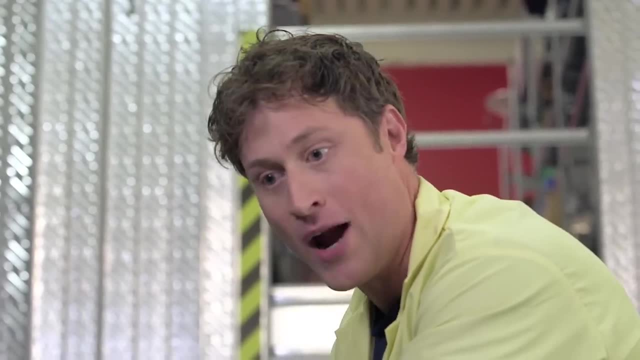 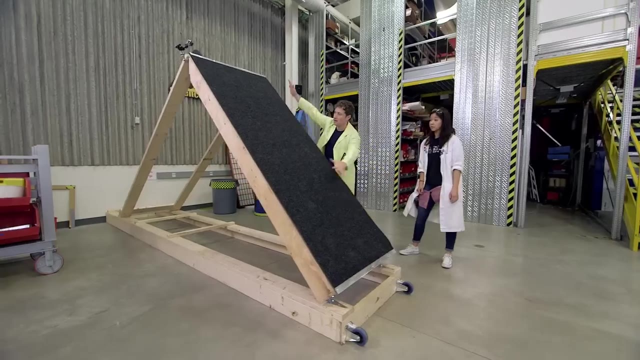 More friction. Let's give it a try. Ha ha, Hey, Way to go, Totally able to climb the ramp. So what do we do now to make it harder? Make it higher, Make it higher. Wow, It's really steep. 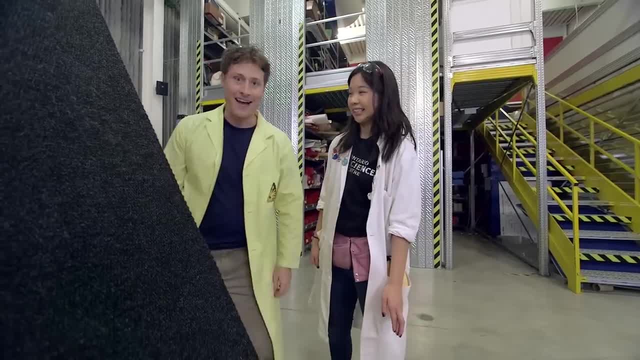 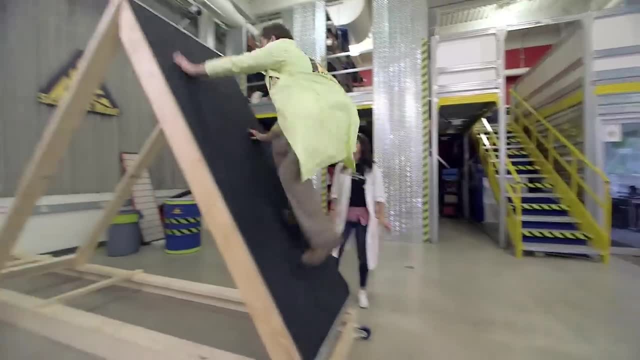 I don't think you're going to make it Sure. If I take a really good run at it, I think I can do it. I don't think so. Well, there's one way to find out. No, No, OK. 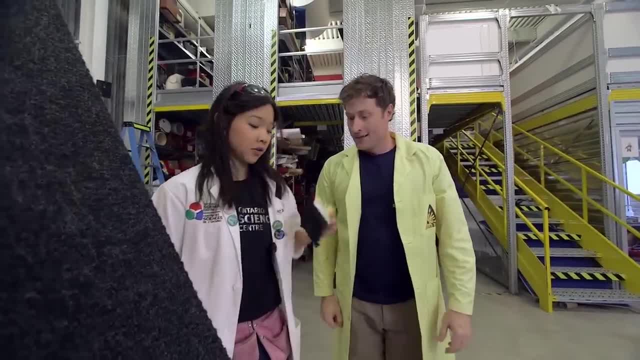 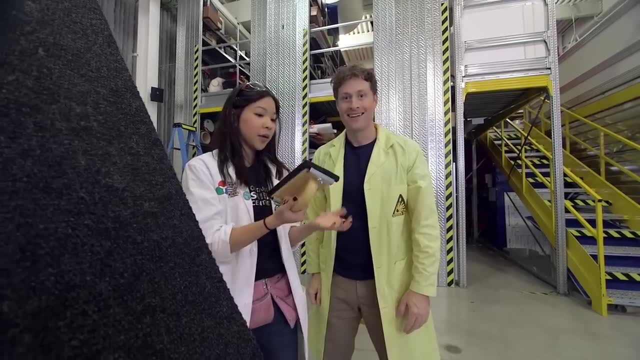 So I can't do it. Is that it? Well, how about Velcro? Wow, Right, It'll give you more friction, So you can try climbing with this. We'll give you Velcro, knee pads, Velcro shoes, Velcro. 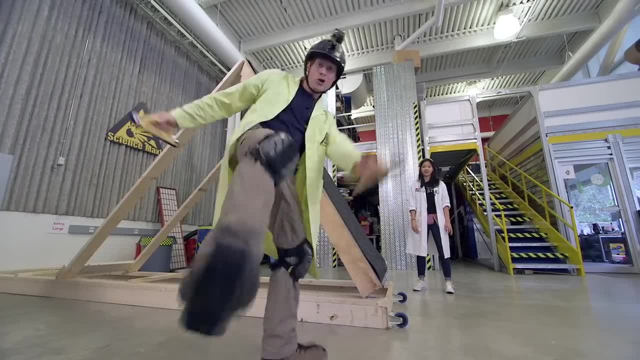 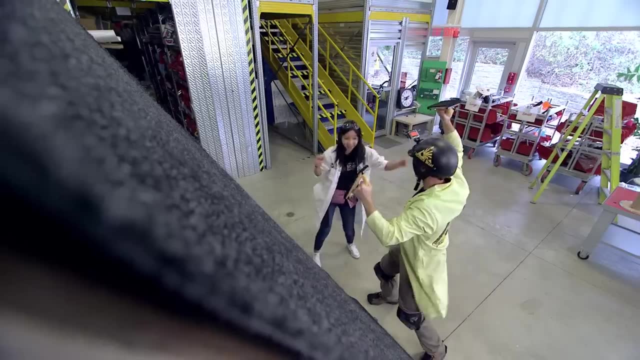 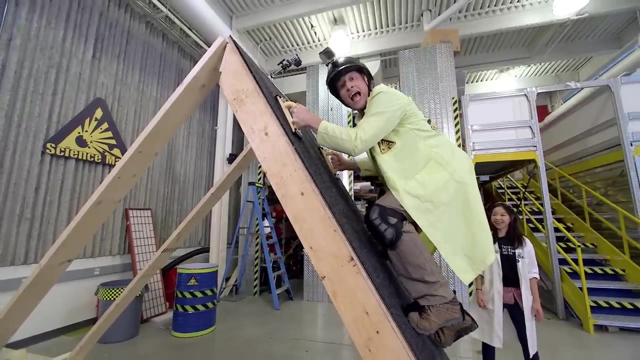 Velcro handholds, Velcro knee pads, Velcro on my shoes, helmet for safety, Velcro fill, Velcro dance. OK, You ready, Ready, All right, Here we go. I did it, Creating friction between me and this ramp. 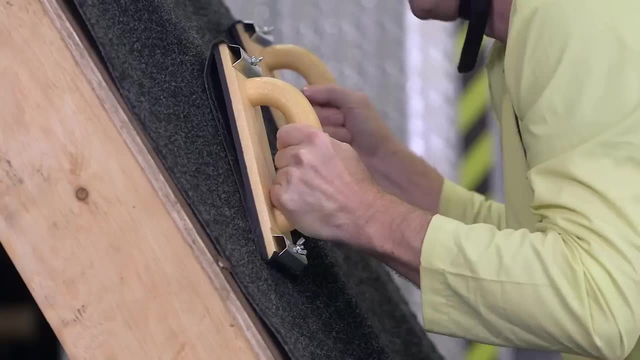 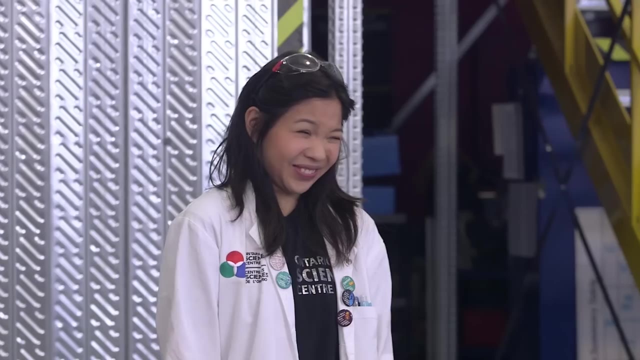 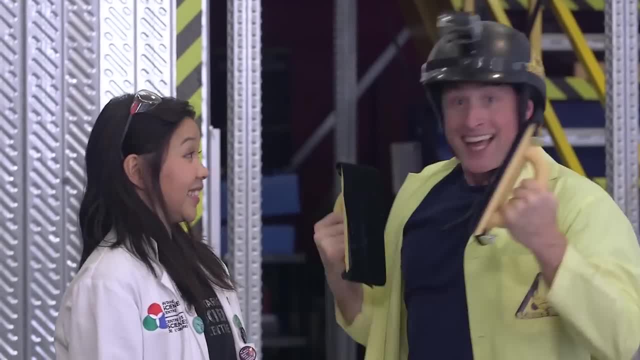 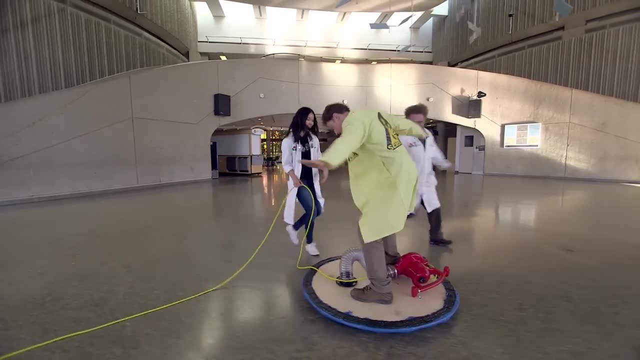 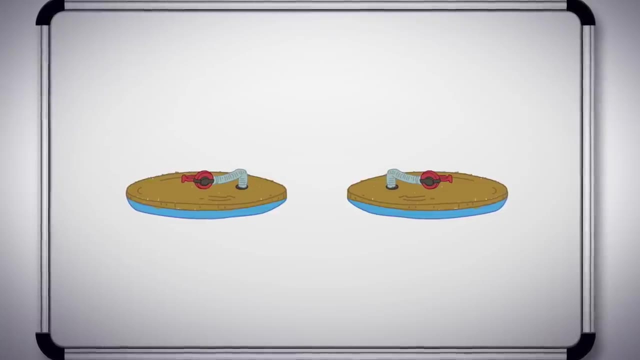 Will you OK? Whoa friction, Your turn. Hmm, Our hover disc worked well, so well that we decided to build another. If we have two hover discs, then we can race them using different kinds of friction to push them along, something that 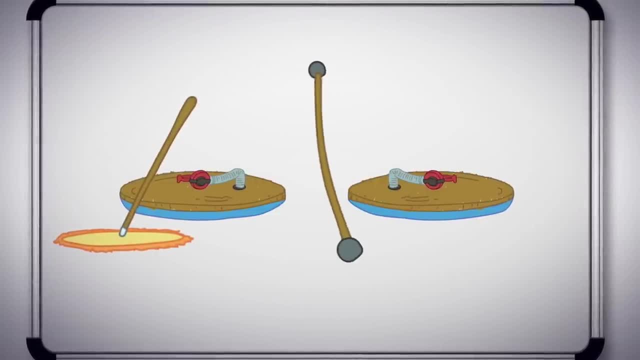 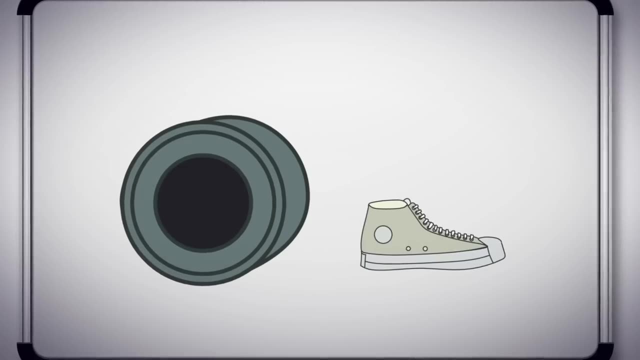 has low friction, like a dust mop, and something that has higher friction, like a pole with rubber balls at the end. That's why we make car tires and the treads of our shoes out of rubber. Okay, we have a giant race course that we've set up. 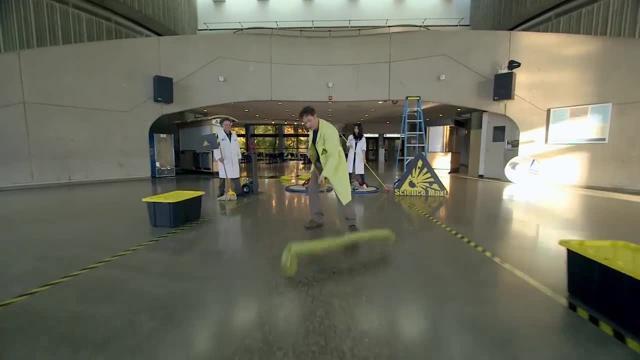 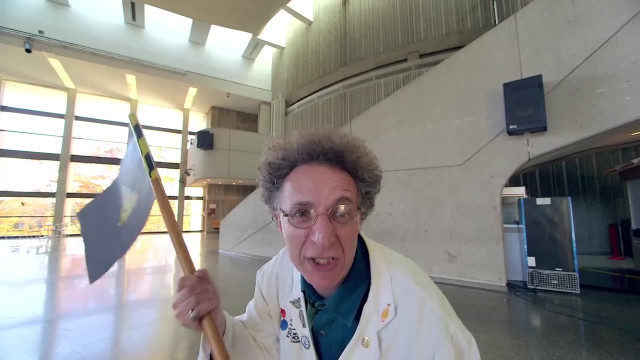 We've got two low-friction hover discs and I'm going to use the low-friction dust mop version to propel my hover disc. And Helena, what do you have? I have the high-friction rubber ball stick. Start your engines. 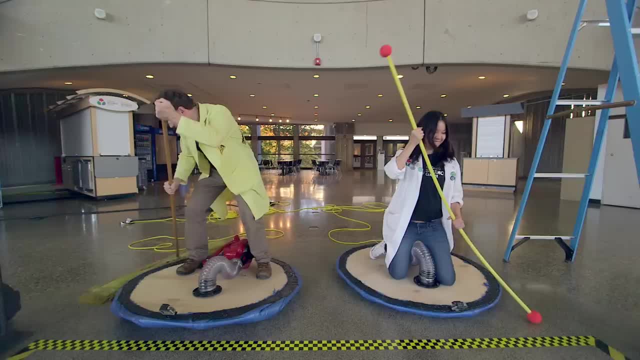 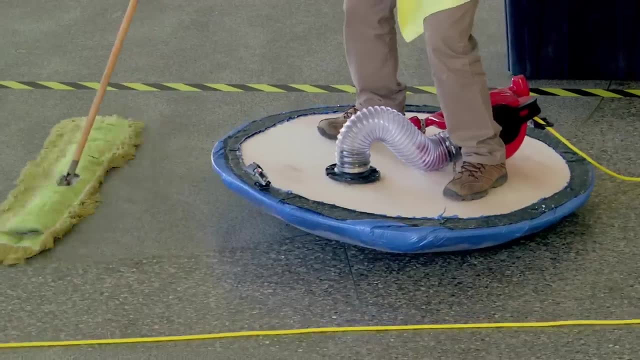 On your marks, get set and go And we're off. Remember, Helena and I are using very different methods to get our hover discs moving. I'm using a low-friction dust mop and Helena is using high-friction rubber balls. 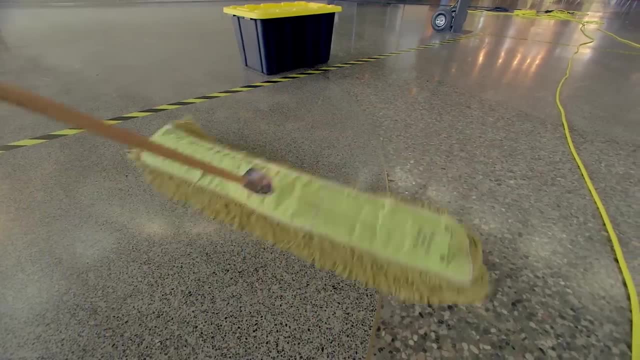 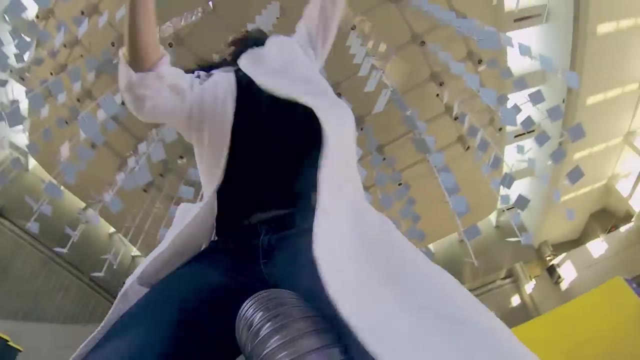 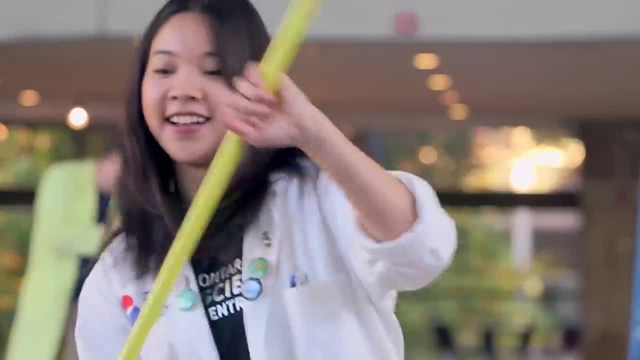 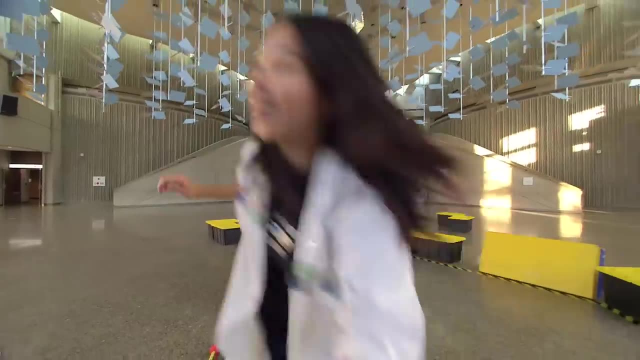 You can beat him Way back. Whoa, Get further, Get further. He's way back over the wind It's a little. She crosses, Yes, And here we have our winner, Yes, Over the finish line and it feels way back over there. 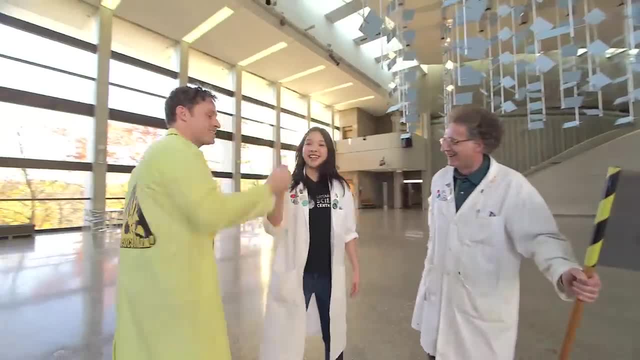 Oh man, I'm still stuck at the second turn. Way to go, Helena, Thank you. So what was the strategy? How did it work? Well, pretty much. while I was using those red balls, I was getting friction helping me steer. 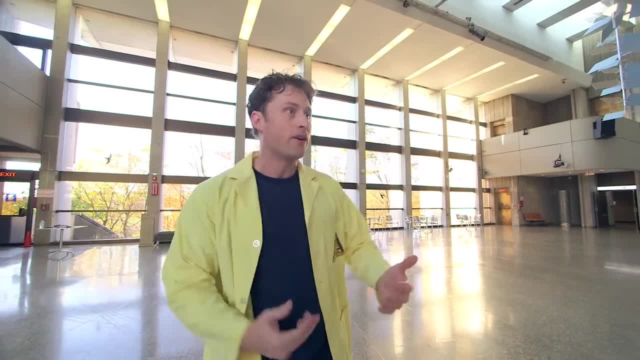 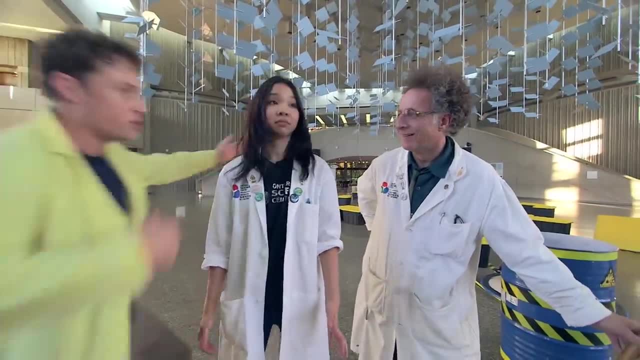 You know what? I think we need a little bit more thrust. That would work even better if we had something pushing us even harder. Definitely, Yeah, Wait, I have an idea. Wait, Hold, Hold, I need your help, Come on. 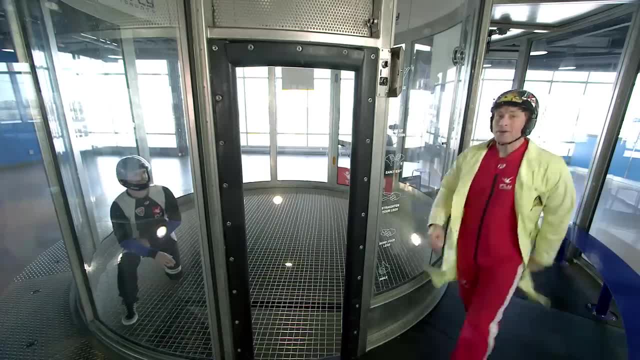 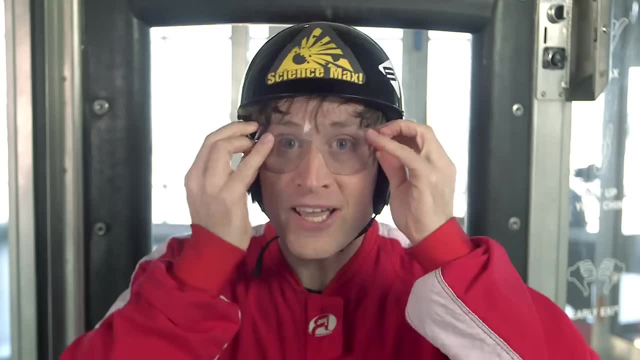 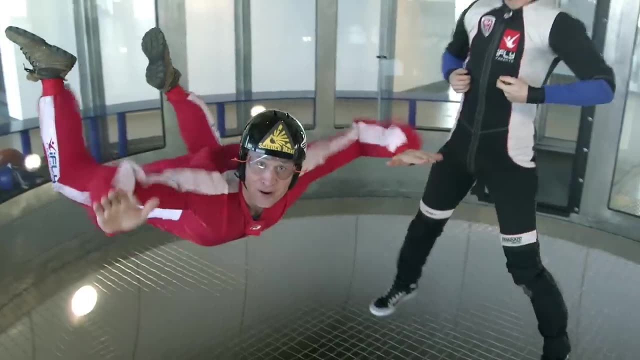 Okay, I'm at iFly Toronto Indoor Skydiving to talk to you about friction. That's Mike. He's going to help me out. Okay, Here we go. What are you going to do? What are you going to think about when we're going through the thing? 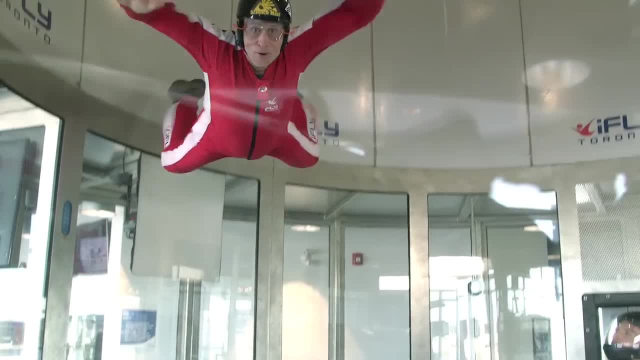 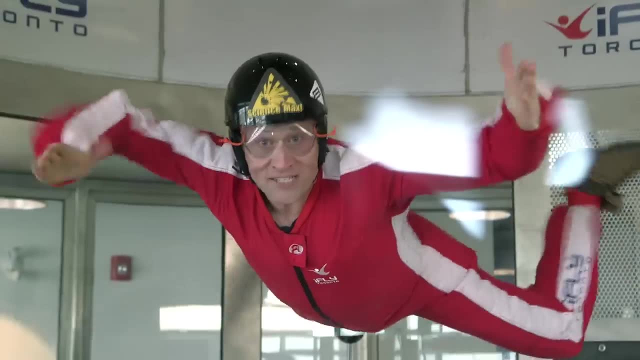 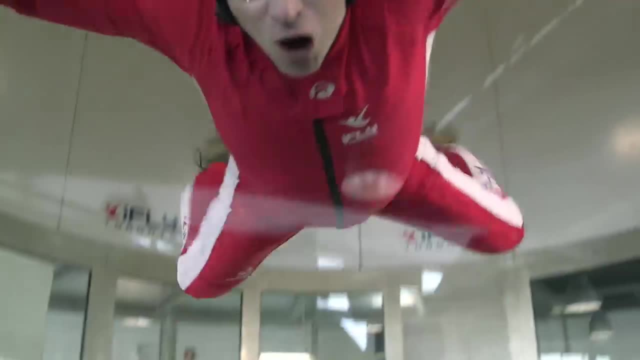 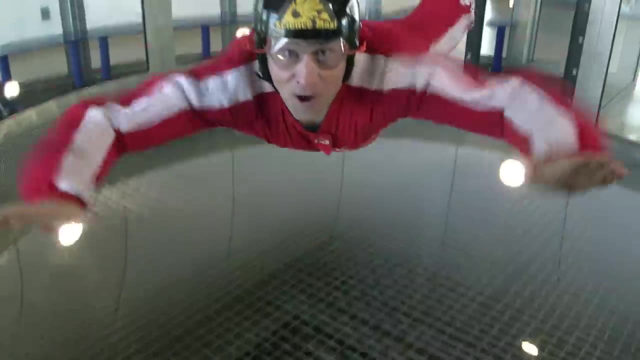 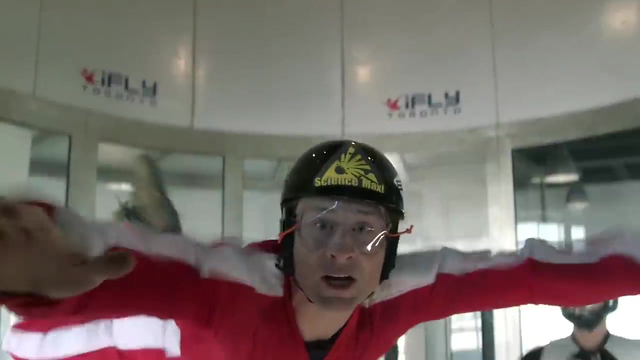 Yes, he's saying. the friction from the air rushing up in the chamber is enough to counteract the force of gravity, which is why he's able to float or swim or whatever he's doing. Now it looks like he might be saying even something like air. 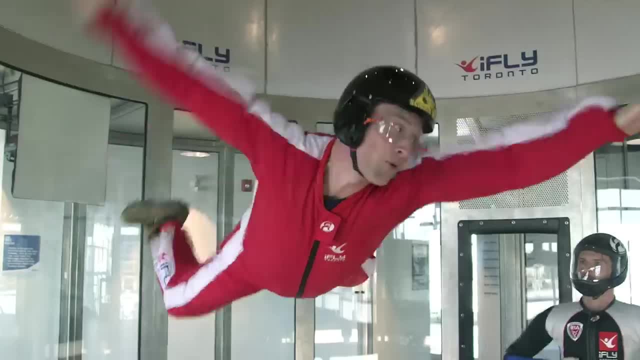 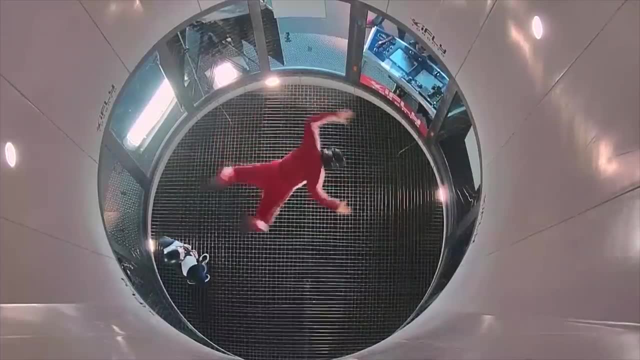 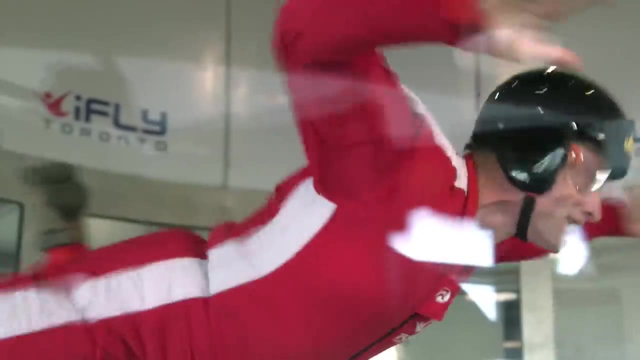 can have a lot of power, Maybe of friction, if it's going fast enough and the air in this chamber is going fast, which is why we can't hear a word he's saying. Oh well, he seems to be having fun. 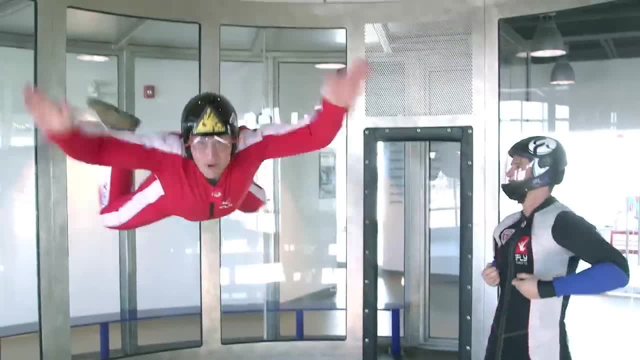 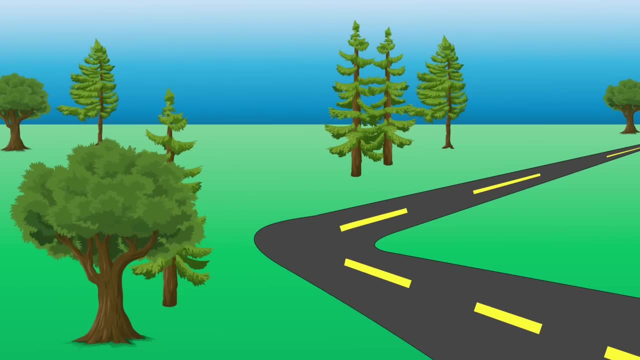 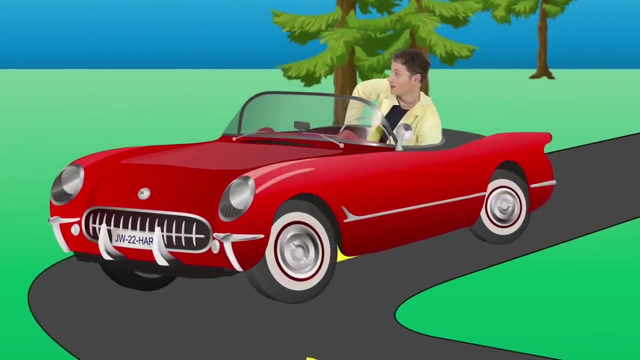 So how important is friction? Well, let's say I'm out for a drive. Car tires need friction to grip onto the road. Without it, my car wouldn't be able to turn At all. But that's nothing. Without friction, the bolts holding the wheels on the car wouldn't work In. 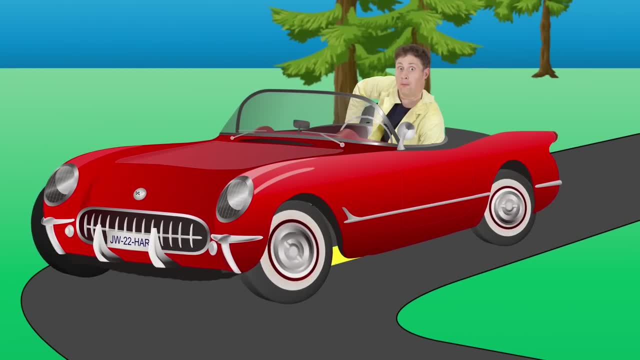 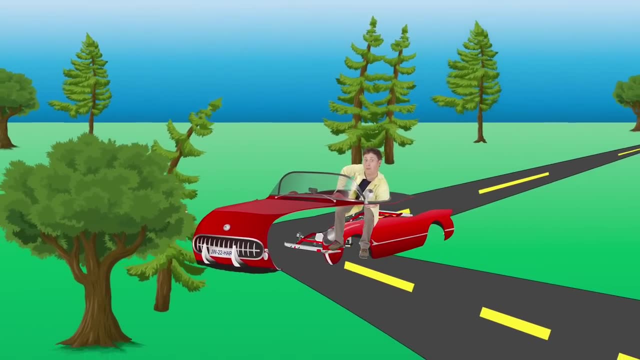 fact, none of the bolts, screws or glue on the car would work and the car would be stuck in the air And nothing would stop moving or stick to anything else. Even the trees would blow away with the slightest breeze. Friction is everywhere And without it nothing. 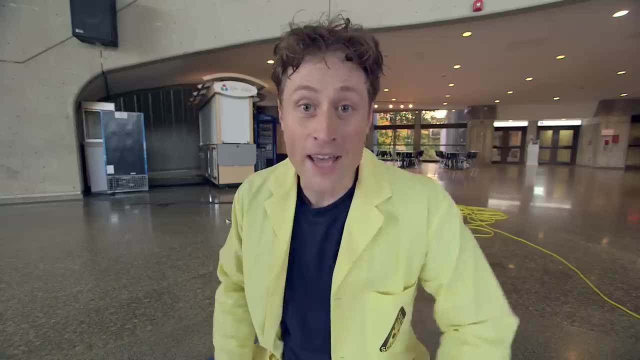 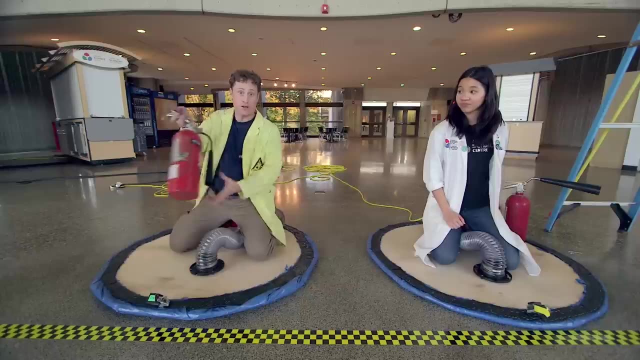 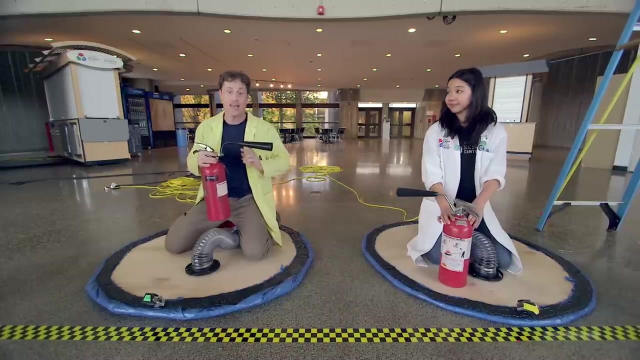 would work. Okay, hover disk race round two. This time we decided to have a little bit more thrust, so Helen and I are going to be using fire extinguishers Now. do not use fire extinguishers at home. Fire extinguishers have a very important purpose and it's not for this, but we 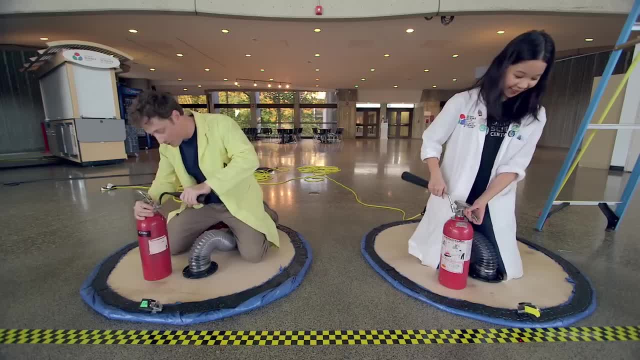 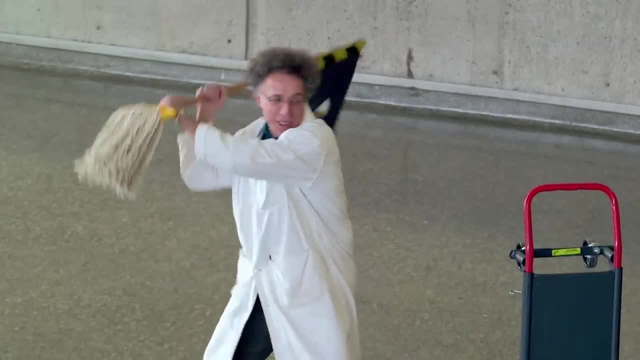 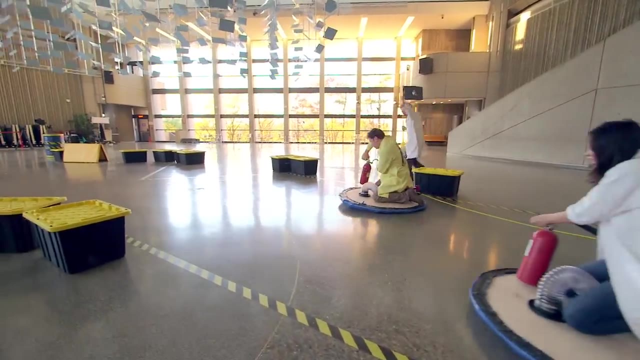 got these ones special. Are you ready, Helen? Oh yeah, Oh yeah. Okay, here we go, Russell, slow Racers, start your engines And go. Using fire extinguishers gives us a lot of thrust, But because the disks we're riding. 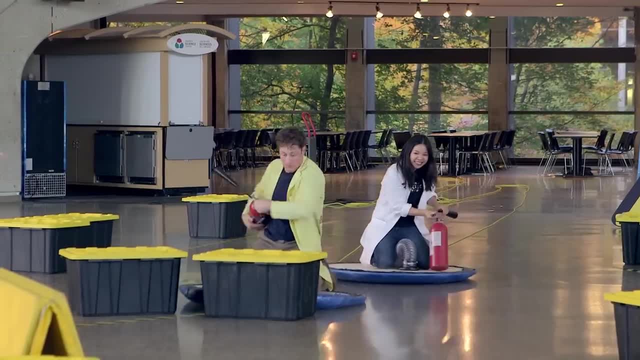 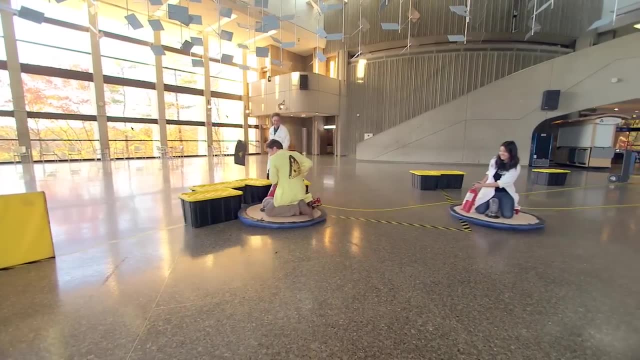 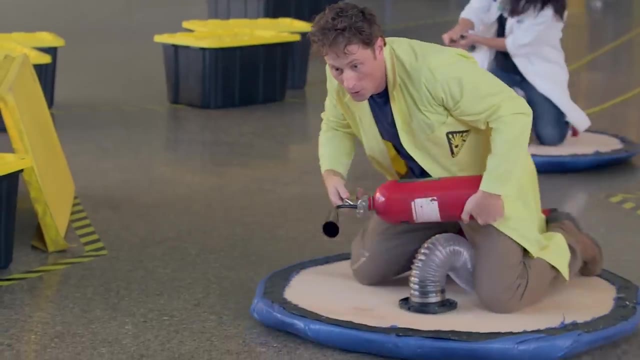 on, don't have any friction. wherever we point ourselves, we just keep going in that direction, Which makes steering very easy. Very difficult. Cars grip onto the road and can go around corners thanks to the friction of their wheels. When you have no friction, it's kind of like moving on an ice rink. 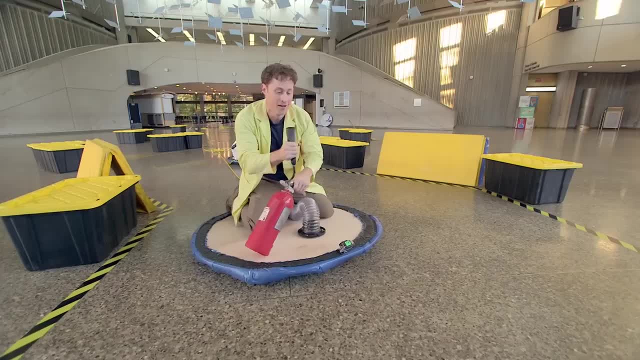 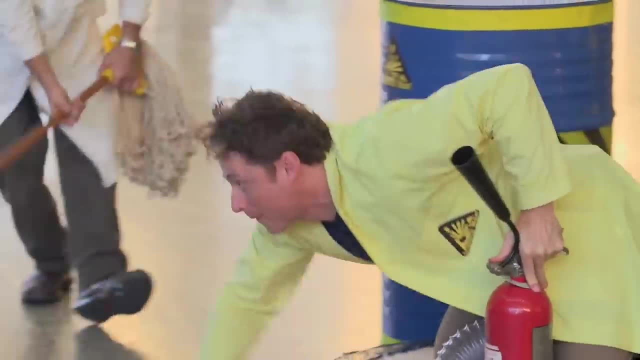 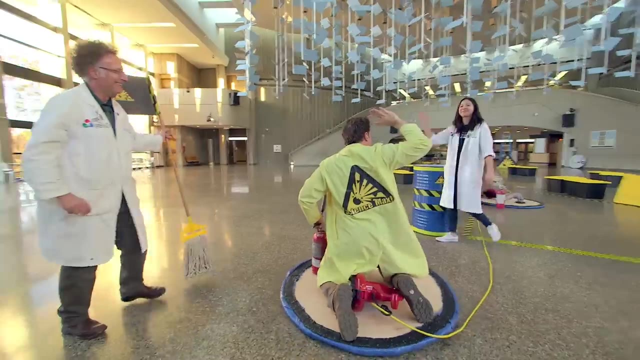 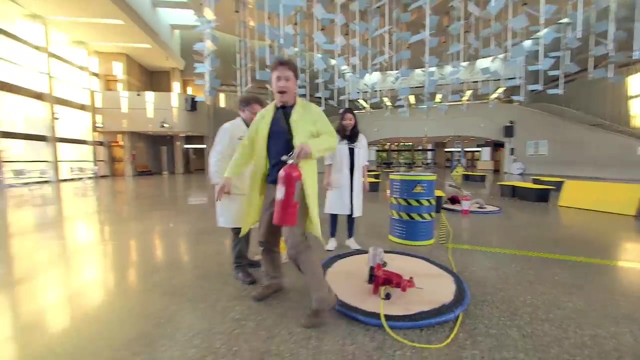 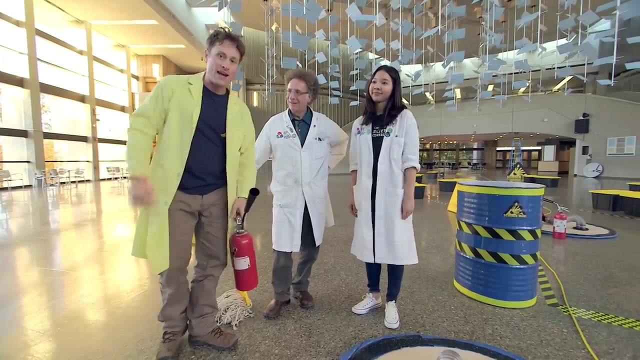 Oh no, I'm out. Yeah, High five, Yeah, High five, Yeah. I ran out of fire extinguisher at the end there, so I had to cheat a little bit. So one for you, one for me and all of them for friction. 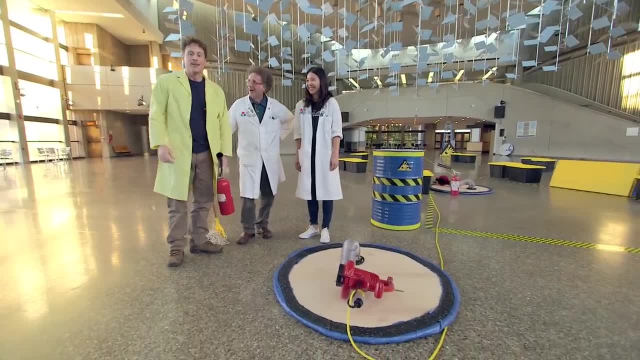 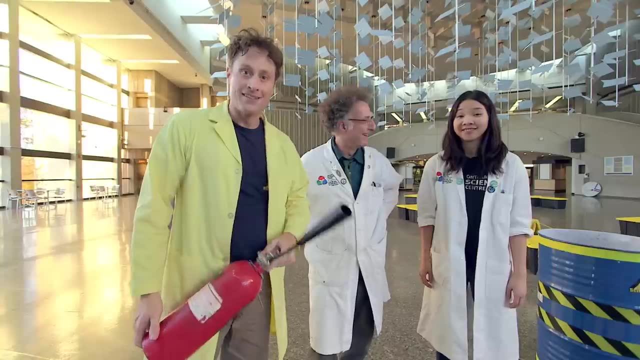 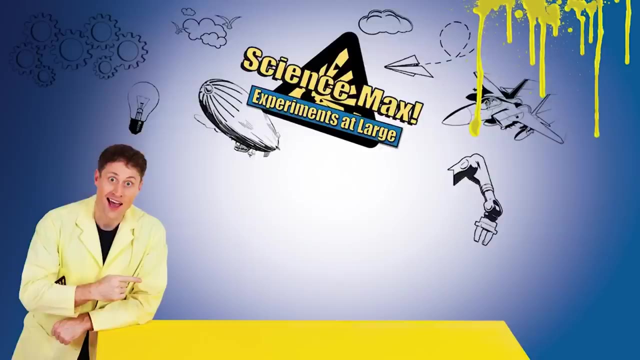 Or the lack of friction, Or the lack of friction? Science Max, experiments at large. What do we do next? Larger fire extinguishers, I think so. Okay, See you next time. Bye, Bye, Bye, Bye, Bye.